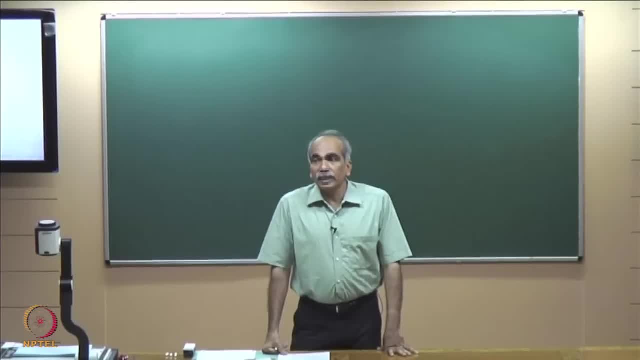 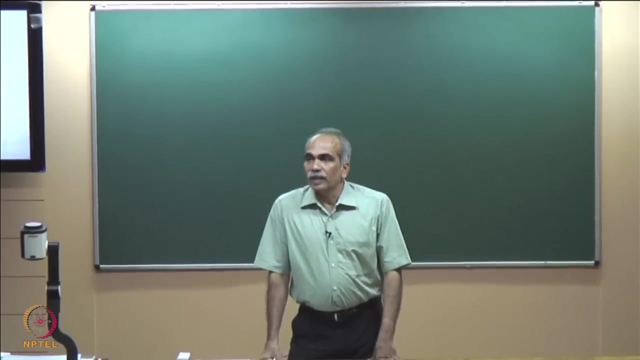 You can also change the conductivity by doping, but at the stage of fabrication there is no real time control on the conductivity, which means if you want to make any switching devices, there has to be real time control. Then we will switch and that is possible by the use of p? n junctions. Therefore, as 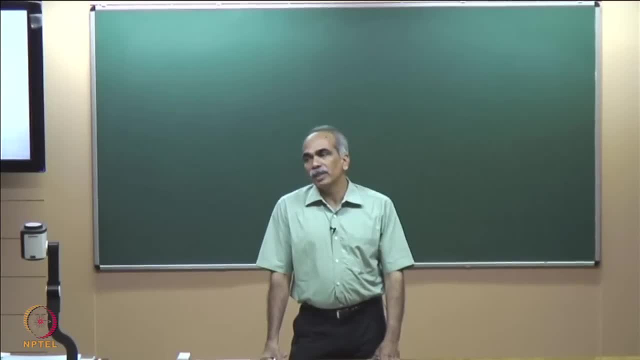 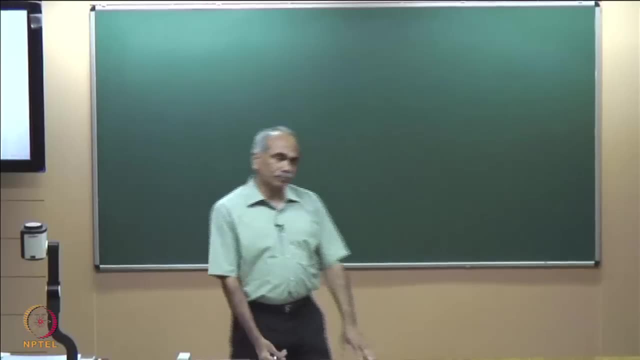 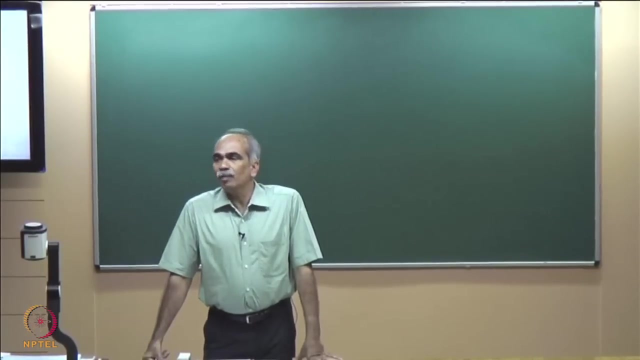 you know, p n junctions form the basic building block of all active devices in electronics as well as in optoelectronics. So my objective would be to recall what you already know about p? n junctions and, in particular, to see how heat row junctions behave or the bands of 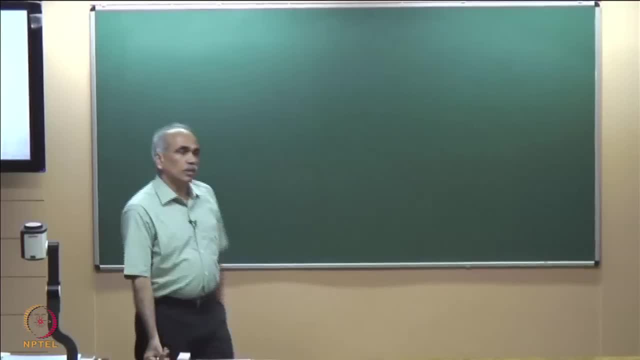 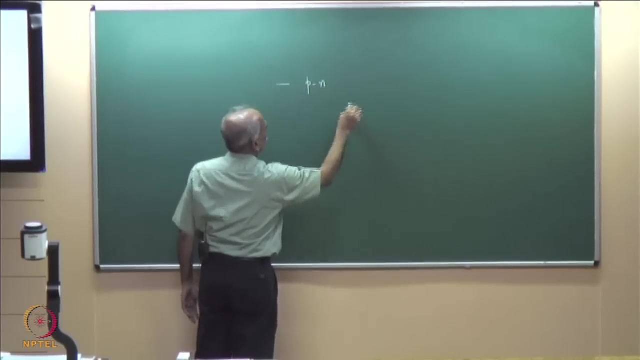 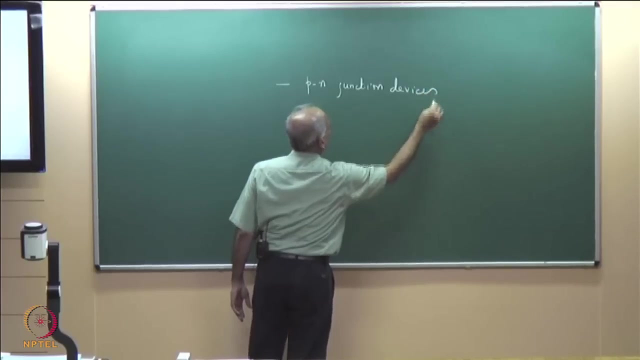 the band diagram of heat row junctions in the case of heat row structures. band diagram of p? n junctions in the case of heat row structures. So the first point is that p n junction devices junction devices for active control, Control of carriers, that is, control of current for active control. The second point is: 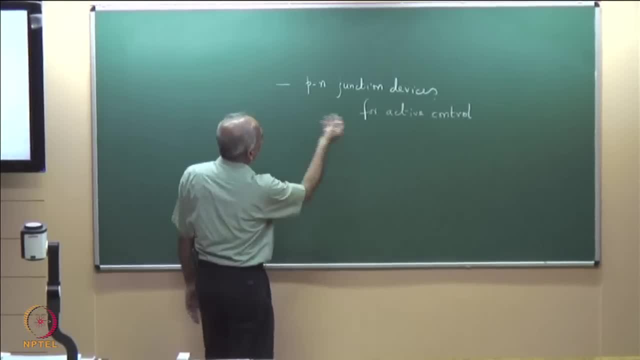 when p n junctions are fabricated or p n junctions are formed. there are usually there are three processes which are used for p n junction. One is diffusion. I have briefly discussed about this diffusion, ion implantation and, of course, epitaxial growth. So this is the process of diffusion of p n junction. So 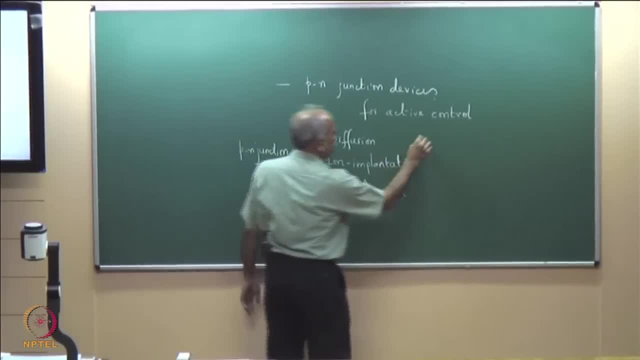 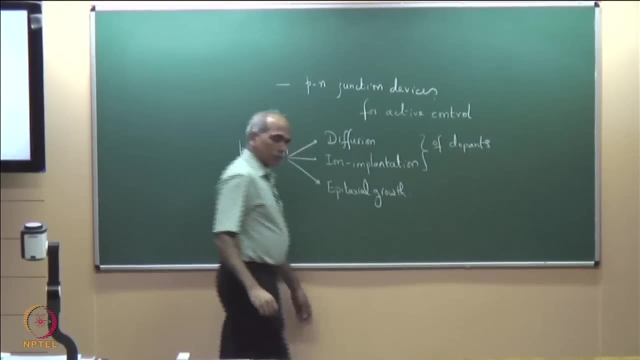 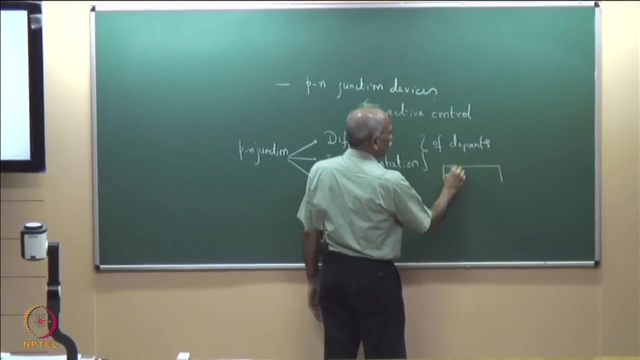 this is the process of diffusion and ion implantation of dopants. of dopants, As we discussed, you start with the substrate and you deposit the required dopant and then diffuse this into the substrate. So this is the substrate. So may be n substrate. So this is the substrate. 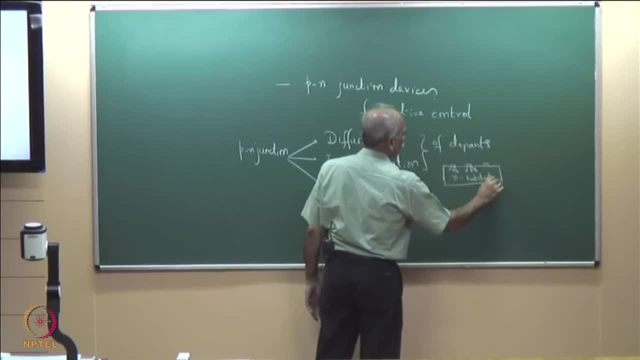 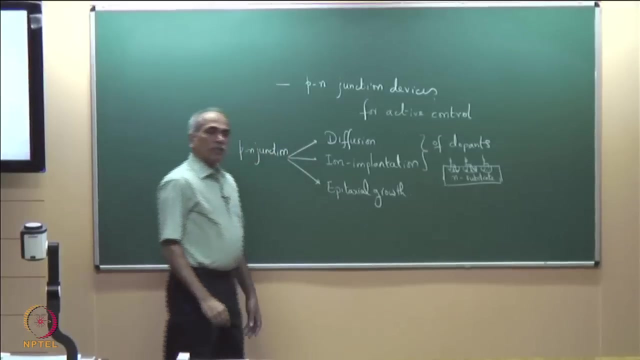 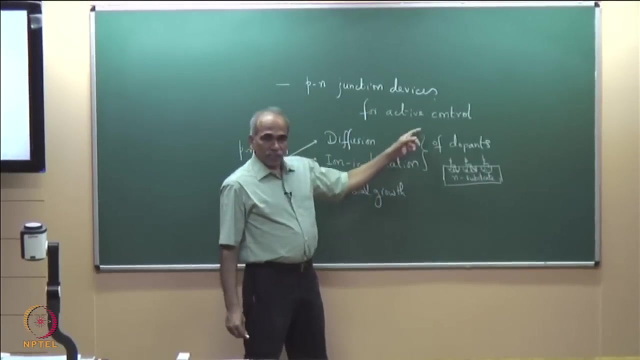 So a little more of the material is deposited and then this forms diffused. the diffused region is primarily p, if you are doping p material. In ion implantation there are ion beams which are implanted into the substrate, But in both cases what you notice, the junction. 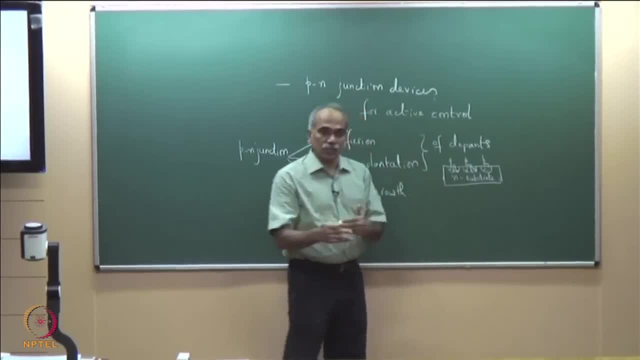 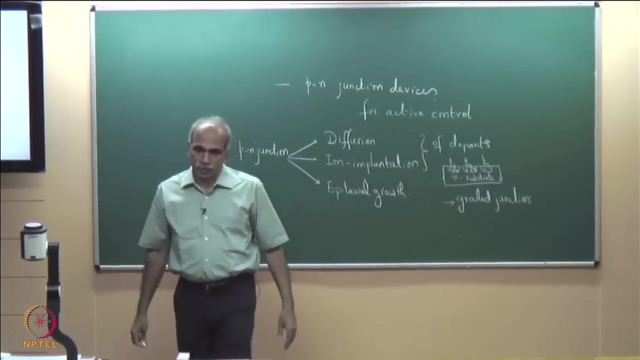 is graded. It is not an abruptcents, So the term is graded. It is not an abrupt substance, an abrupt junction, it is graded junction. So both the processes lead to graded junctions: graded in terms of carrier concentration, in terms of dopant concentration, But epitaxial. 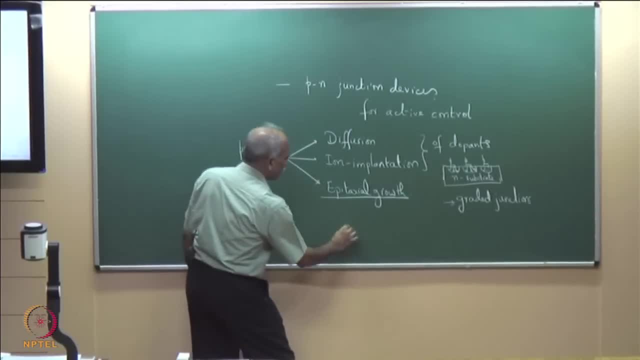 growth. in epitaxial growth- we have already discussed in detail- you start with the substrate- let us say n substrate- and then you do: you deposit a layer, may be n plus. or you deposit a layer, let us say p, then the junction is really abrupt, In other words, the typical. 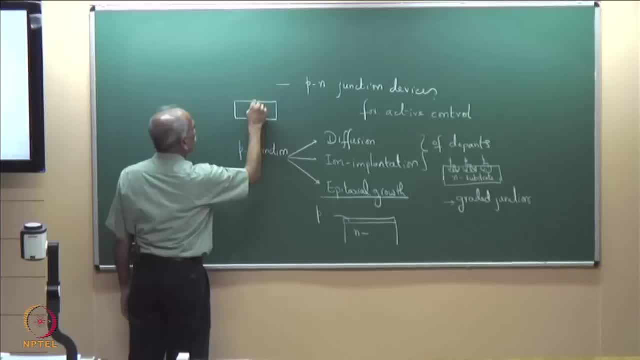 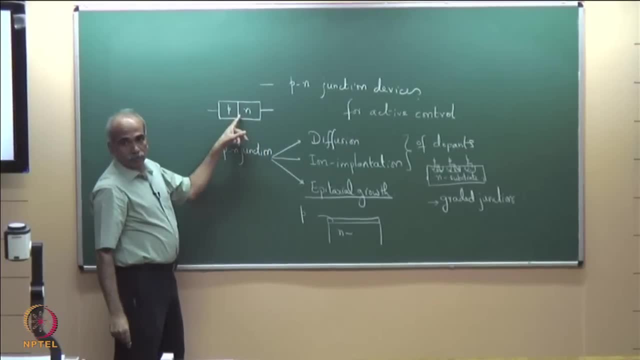 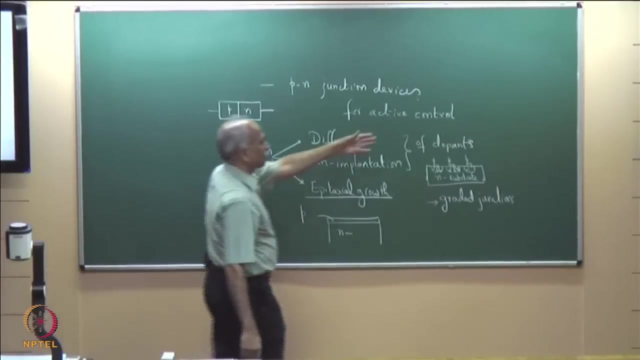 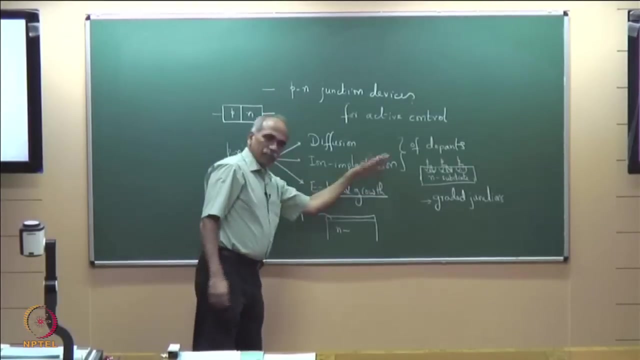 p? n junctions that we show, like this schematic which we represent: p? n. this is an abrupt junction device and by epitaxy, indeed, you can grow So abrupt junction devices. otherwise these processes normally lead to graded junctions. Both have their advantages and disadvantages we will discuss, probably at a later stage. 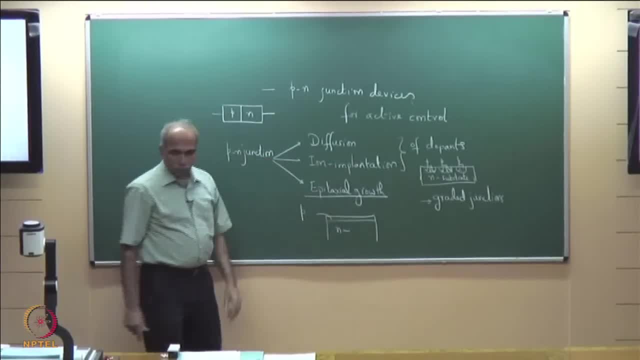 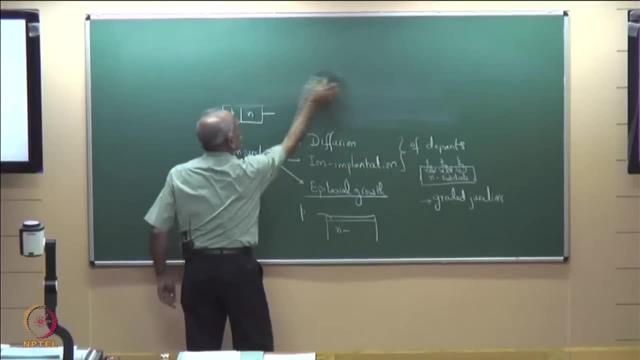 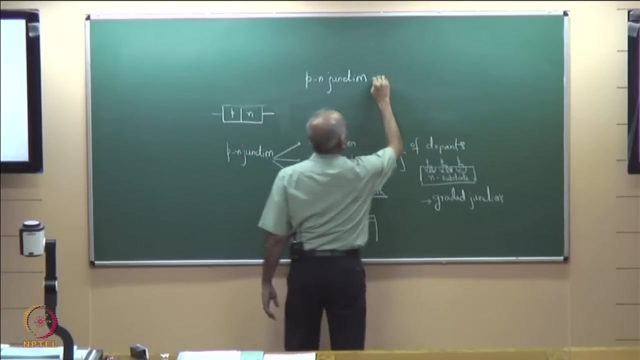 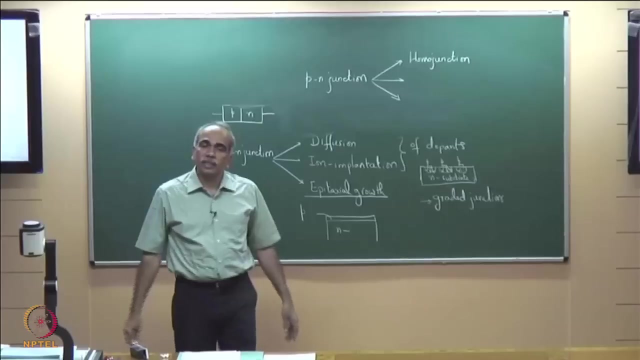 but this is regarding the growth and type of p? n junctions in terms of material and structure. The second type, second type of classification here, is homo junction, that is, junction between same material but p doped and n doped material. P type silicon. n type silicon. hetero junction: junction between dissimilar materials. hetero junction usually with the different band gap and also Schottky junctions. This is junction between metal and a semiconductor. When you make the device finally you need metal layer. 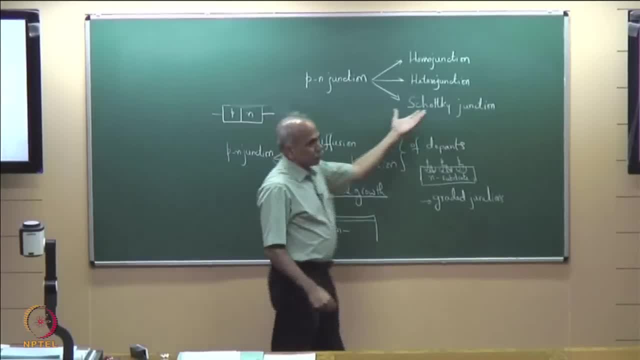 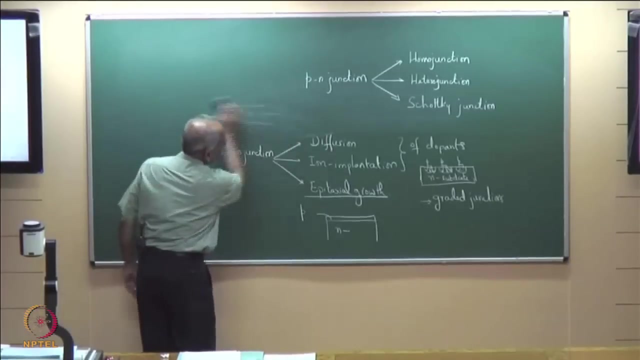 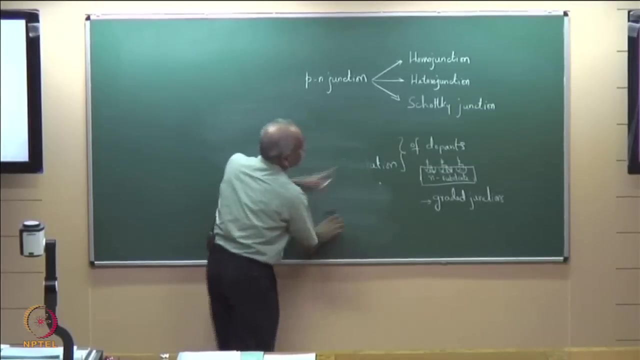 for contact And you will always have a Schottky junction and we will see how Schottky junction, Schottky junctions- can behave, both as rectifying junction as well as ohmic contacts. That will be our next discussion. So this classification was based on process and this classification is based on structure. 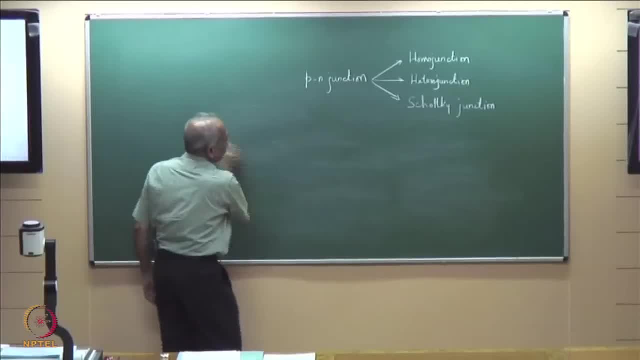 So let me quickly recall the band diagram, the energy band diagram. So energy band diagram of p? n junctions. A band diagram is basically the energy band diagram of p? n junctions, The energy band. We have a p-type material, So this is the p-n junction, p-n, So metallurgy contact. 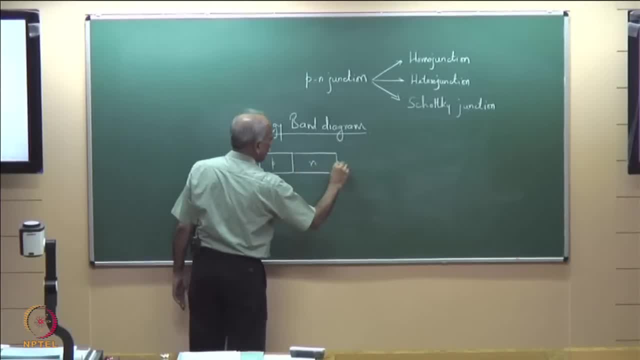 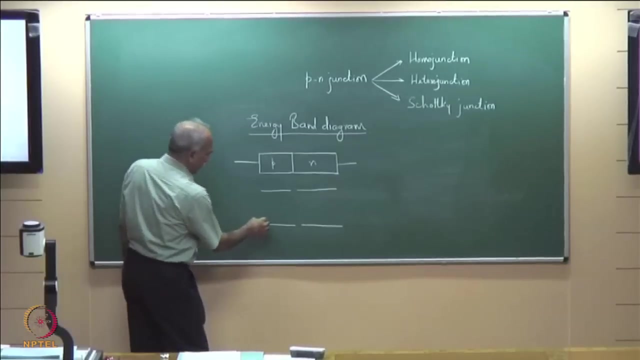 p-n, p-type material, n-type material. and if you draw the- let me first discuss- homo junction, If you draw the energy band diagram before contact, p-type will have Fermi level somewhere here and n-type has Fermi level somewhere here. So this is p-type and n-type. 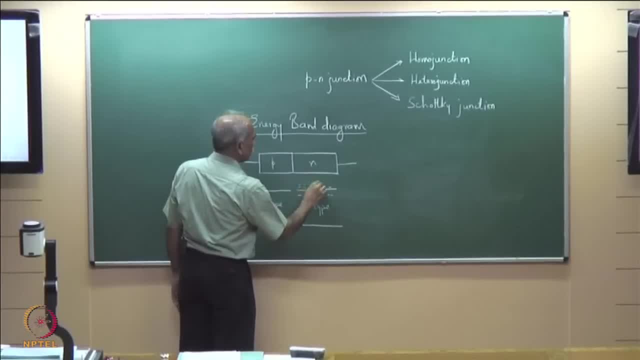 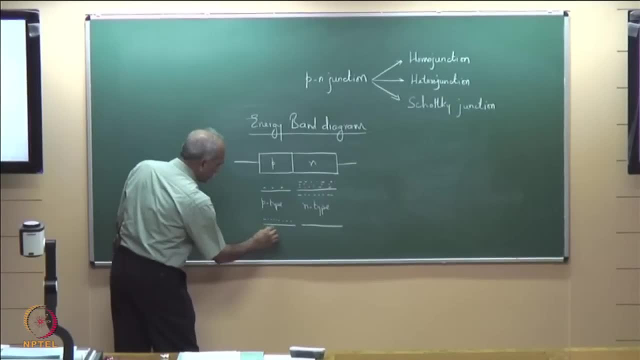 It tells me that there are large number of electrons here in the conduction band, a very few electrons here. There are large number of holes here and very few holes here. So when you form a p-n junction, naturally there is a difference. 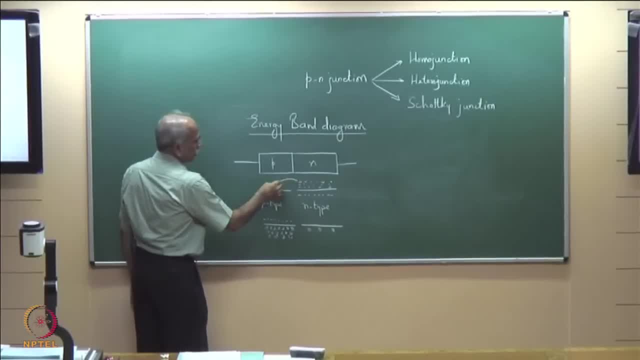 in carrier concentration. So electrons when you form junction, electrons diffuse from high concentration, So from high concentration region to low concentration region, and holes diffuse from this region, So there is a diffusion current. So electrons are moving in this direction, which means 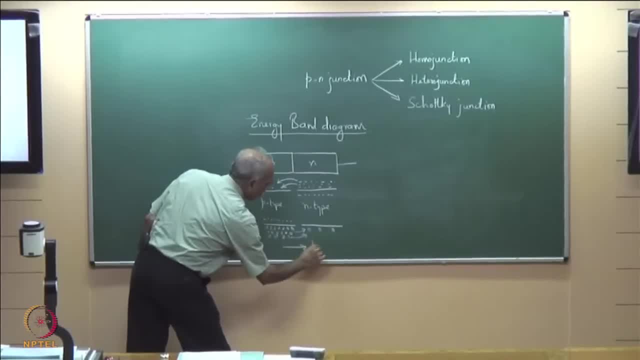 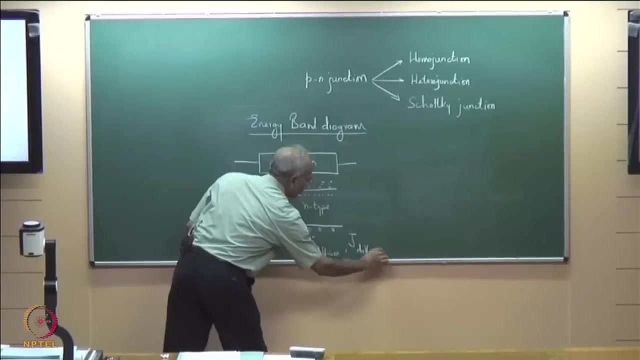 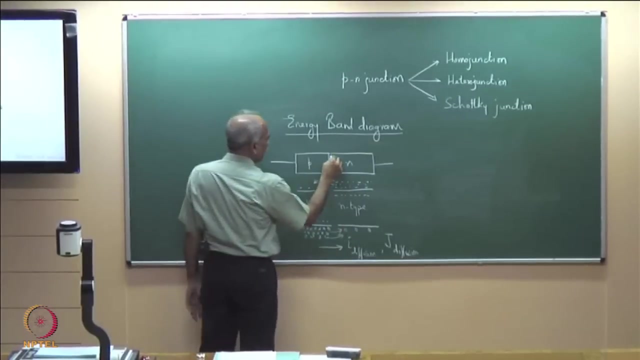 we have a diffusion current, I diffusion, So I diffusion, I diffusion, or A, J diffusion current density, g diffusion because of difference in carrier concentration. At the same time, when electrons move over to this side or holes move over to this side, this leaves behind immobile ions. 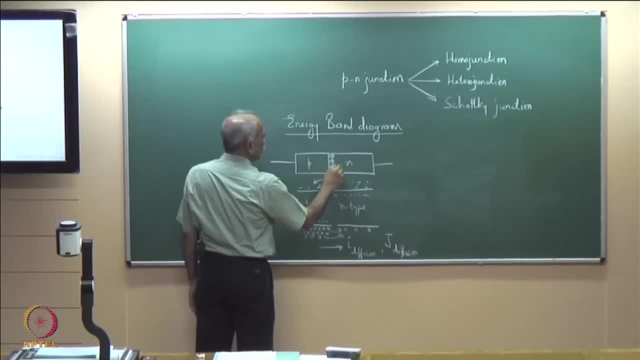 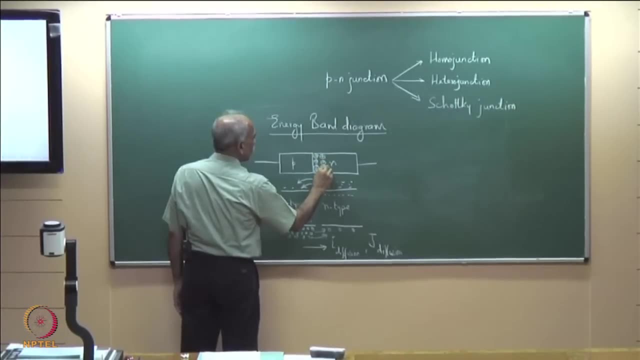 positive immobile ions- all of you have studied this, I am just recalling- and negative immobile ions here because holes have moved. So these are negative immobile ions. the depletion region and therefore there is a we have built in potential here, potential difference which leads to drift current Whenever. 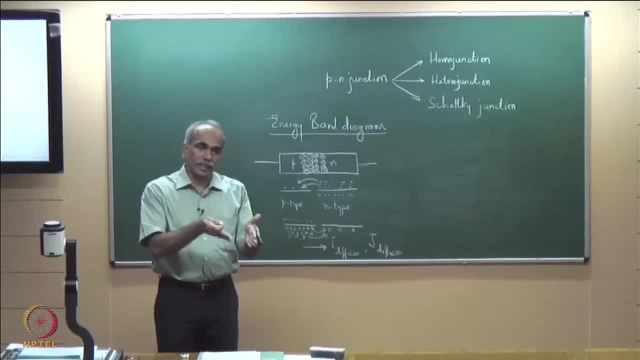 you have a material where there is a potential difference and if there are carriers, then there is a drift current. So the drift current will be from positive to negative. So I drift drift current refers to the current in the presence of an applied potential difference. 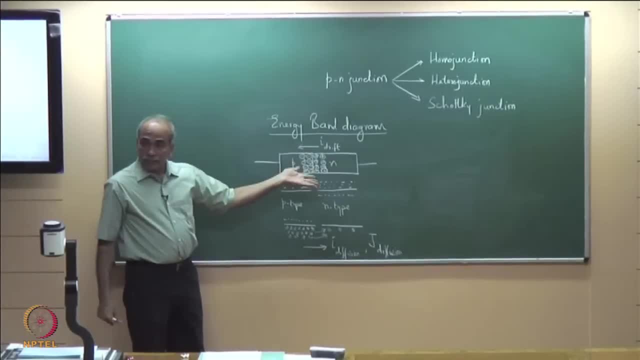 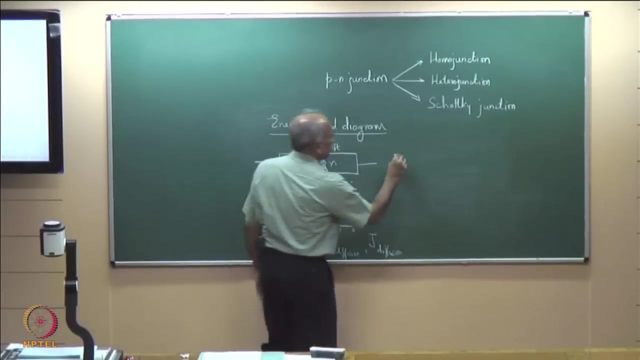 So there is a drift current because there are always minority carriers in the drift diffusion region and this leads to a drift current in this direction. So there is a diffusion current and there is a drift current at equilibrium I diffusion, So J diffusion. 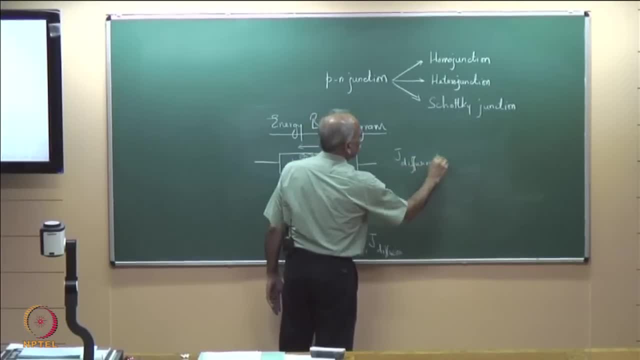 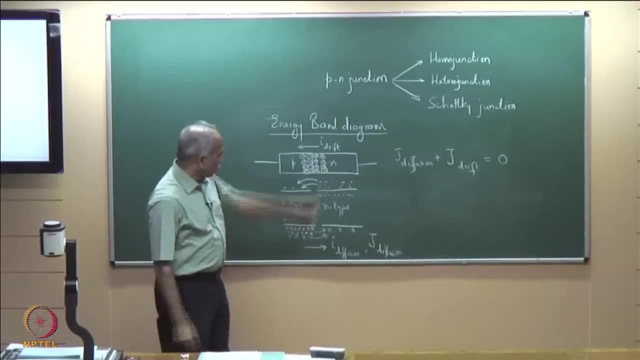 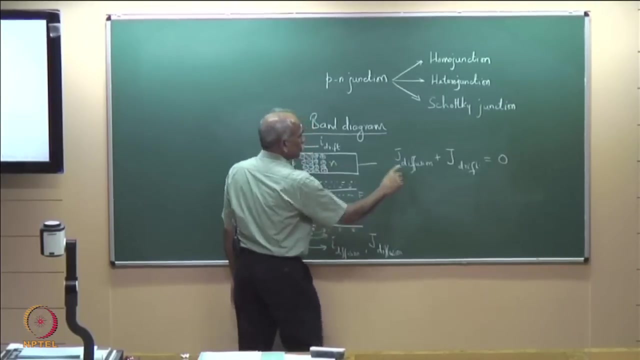 plus J drift equal to 0.. Mathematically you can show that this corresponds to: if you have EFP here And EFN here, you can show that this implies d, EF by dx. I am showing one dimensional x direction- dx equal to 0.. This implies- this is pure mathematics and this shows that EF is independent of x. this 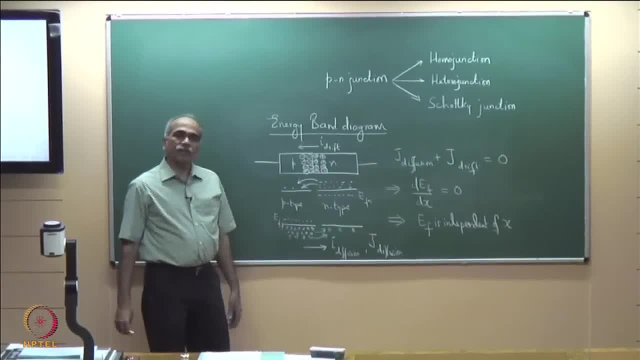 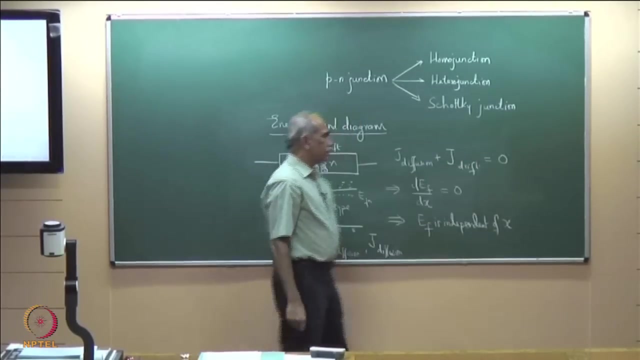 is a one dimensional dimension. picture x is in this direction. E F is independent of x, which means E F remains constant, So at equilibrium. so the drift current, essentially equivalent to diffusion current in magnitude and in opposite, in sign. that is why it is 0 and we have all done this. 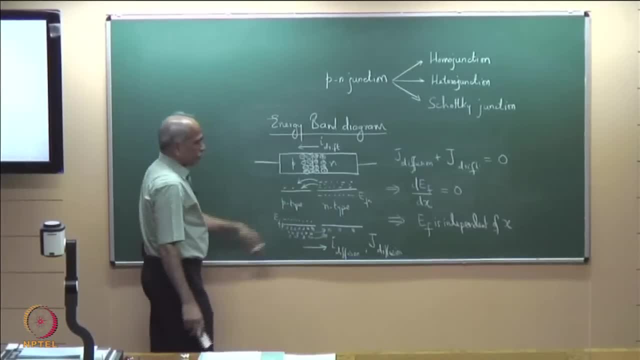 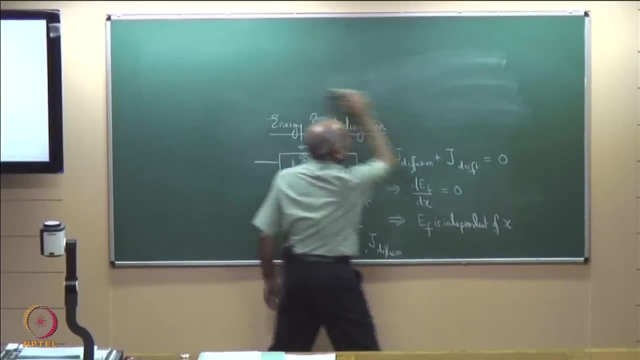 that you can show that E, F is independent of x. that means the Fermi level is constant throughout: 0, 1, 2, 3, 4, 5, 8, 5, 16. The band has to bend which way the band will bend, whether this will go up or this will. 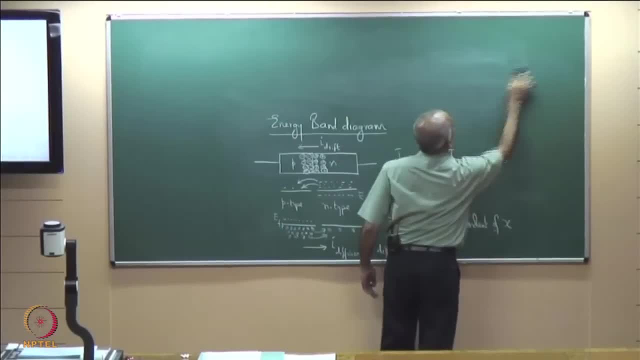 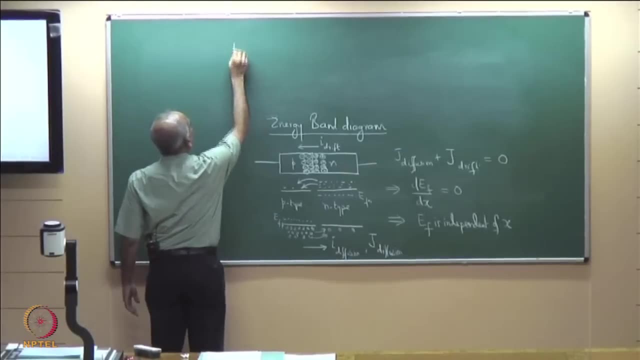 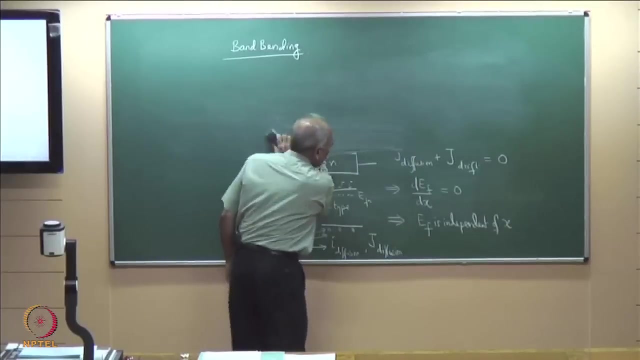 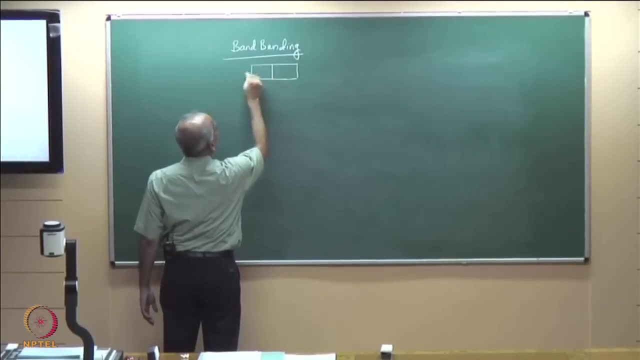 come down we will see which way the band will bend. So let us look at this again: band bending From elementary. let me redraw these. Let me draw here p-type and n-type. I will show a little wider depletion region, so you 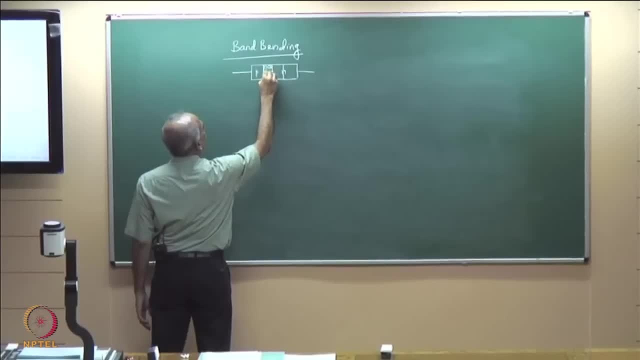 have negative immobile ions here. it is a quick revision because this is important for us: to see the band bending in hetero structures. that is why I am just repeating: all of you are aware of this. So there is charge distribution here and therefore we use 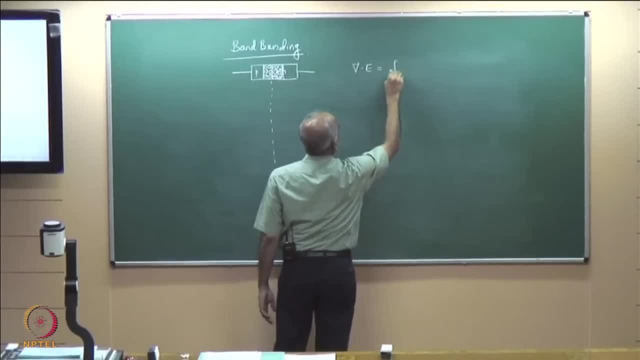 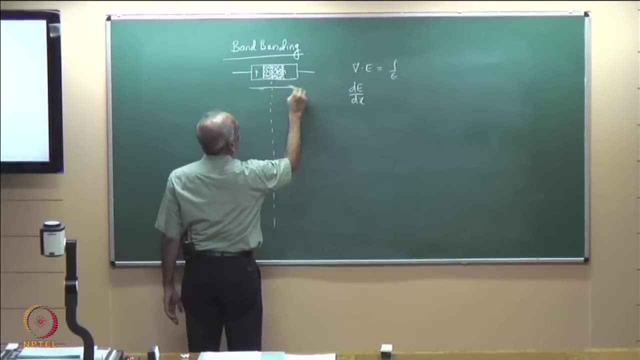 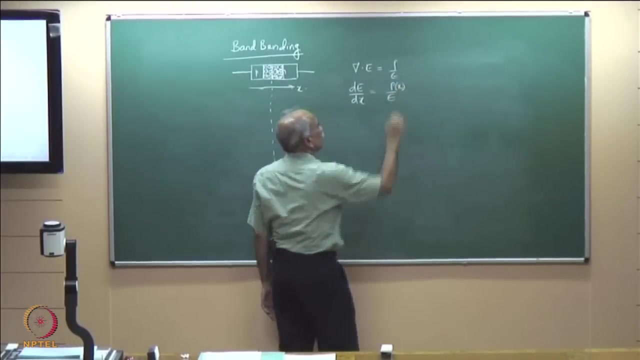 this Gauss laws del dot, e is equal to rho by epsilon, or in 1 dimensional I can write d: e by dx. x is this direction, de by dx is equal to rho by epsilon. rho is the carrier, density, charge density. So this is rho of x in one dimension. actually rho is volume density, but in a 1 dimensional. 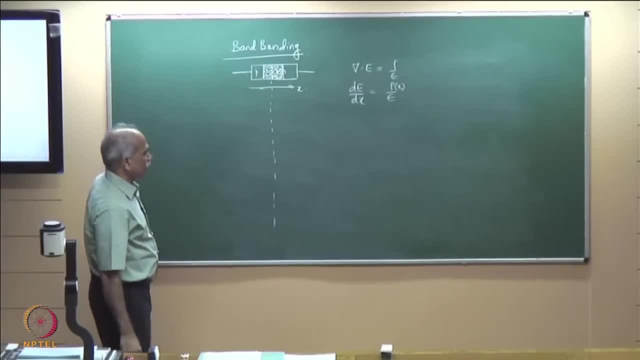 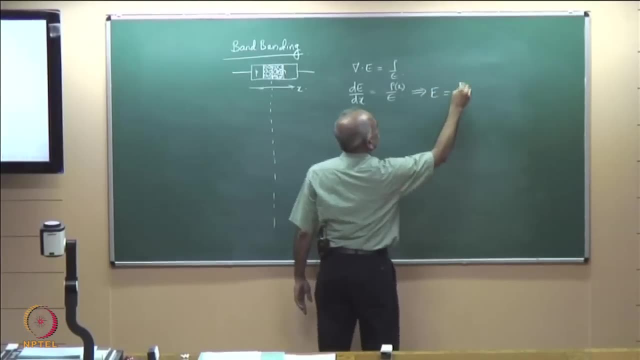 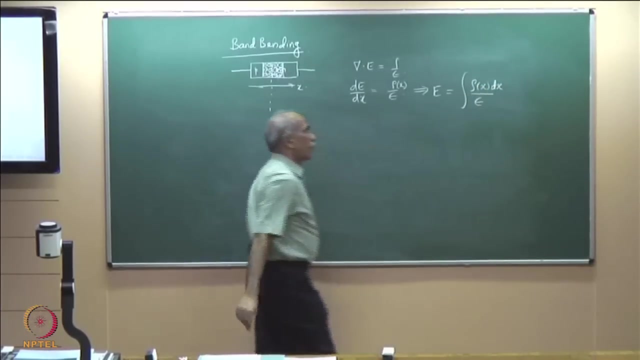 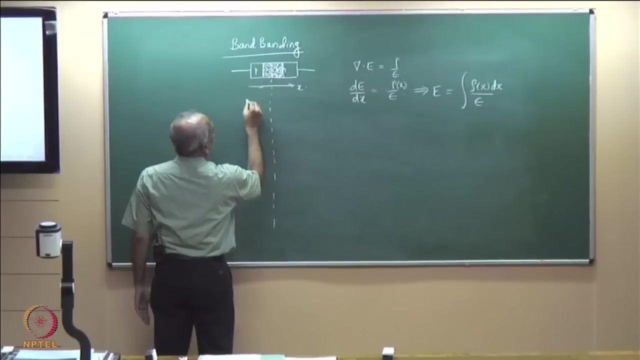 simple picture: d by d. x is equal to rho of x by epsilon, which means this implies E, the electric field. E is equal to rho of x, d, x by epsilon. It is a simple integration. So we have. so if I want to plot rho of x here, so this direction is x, rho is negative here. 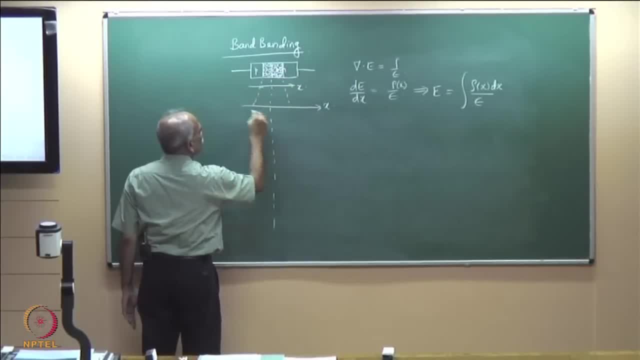 I assume that. so, corresponding to this. so there is negative rho of x and positive rho of x. So what I have plotted here is rho of x. This is rho is negative, negative charges and here positive charges. So this is rho of x. The electric field, if 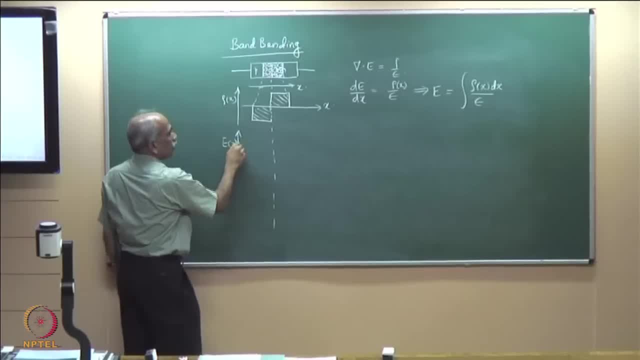 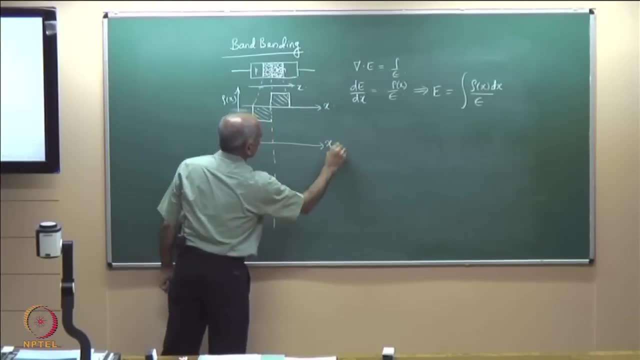 you plot the electric field. now, E of x is simply integral rho of x, d, x. So again plot x. beyond this there is no electric field because the charge is from here. So electric field is integration. So it is integration and adding rho of x, d, x. So you are going on. 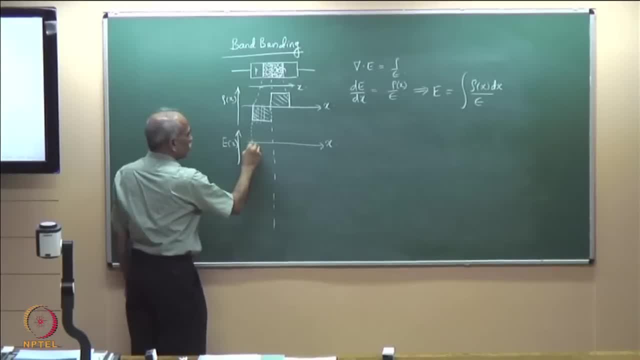 adding segments like this: rho of x, d, x, which means it will increase as a triangle summing up different segments. So it starts from 0 here and then rho is. So you are. it is negative because rho is negative. So this is 0. this is negative. 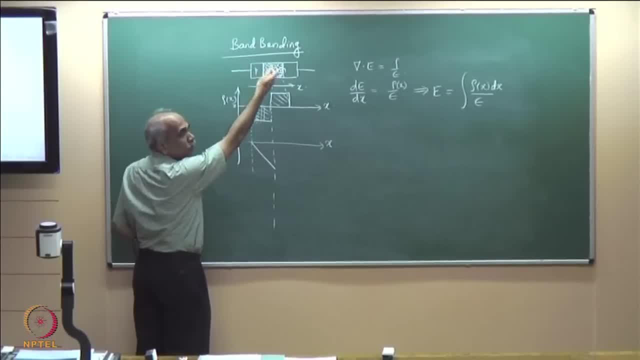 I have assumed. I have assumed that there is a constant distribution, uniform distribution, normally in an abrupt, normally there is a little bit of gradient, but for simplicity I have assumed a uniform distribution. So when it comes here it is the you have added area which is all negative. 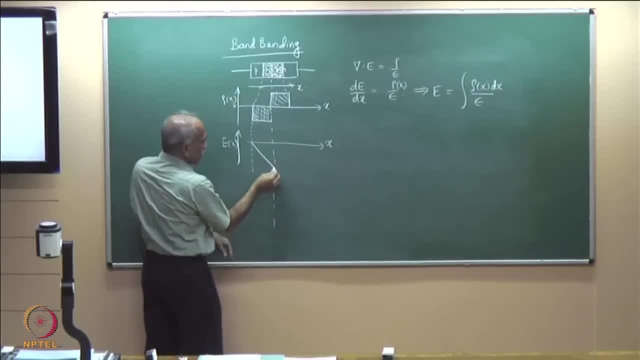 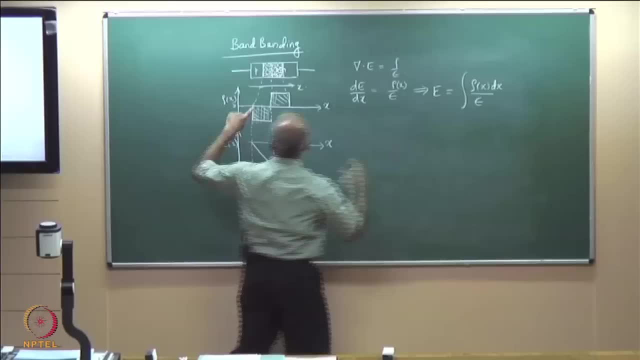 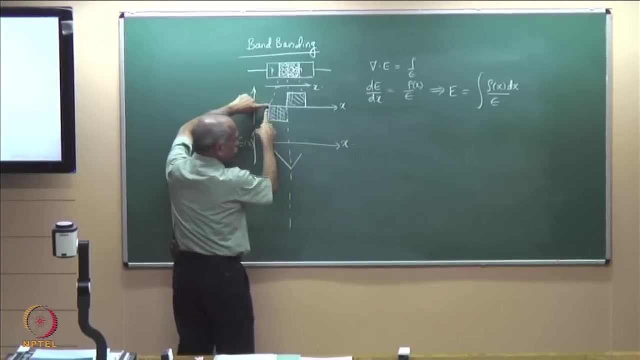 now you add positive part of it, which means the sum will decrease, So the sum starts decreasing. please see, integration continues, So the electric field continues from this end to this end and finding out electric field everywhere. there are no charges here, So charge first starts from here, So electric. 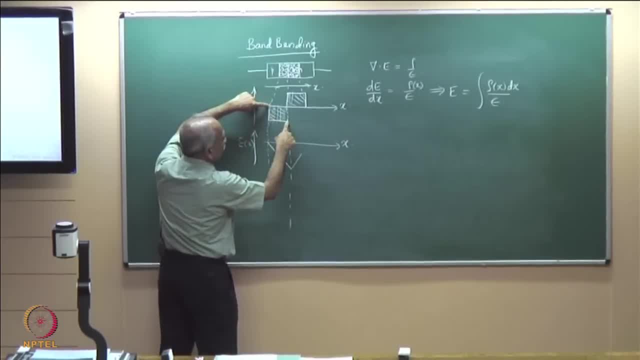 field is negative, like this it comes. you have added up to this. then you are adding positive to a large negative number. So the negative number is decreasing and therefore the electric field is decreasing. So the electric field comes down to 0.. So this is electric field. 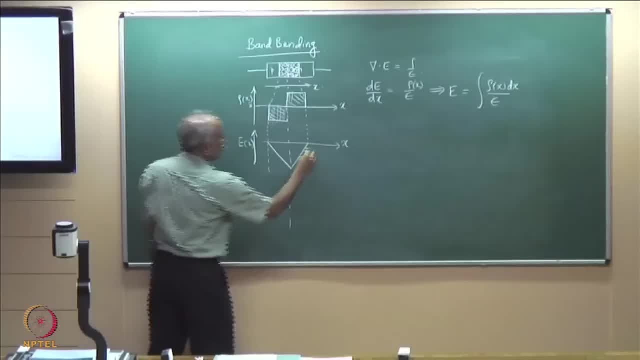 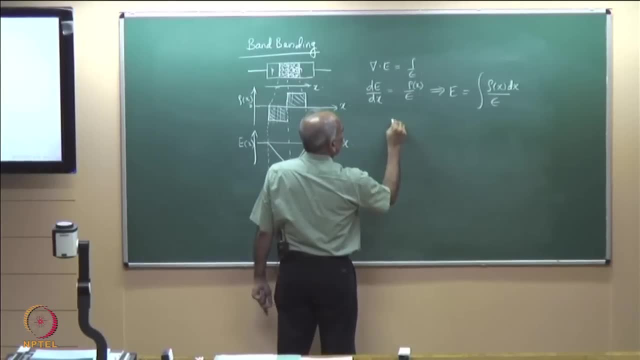 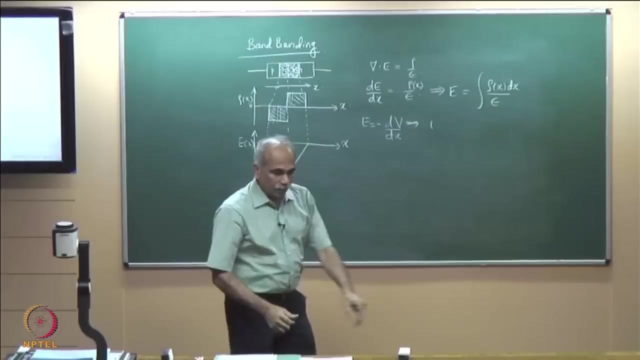 variation. from this end to this end. there is no electric field far away from the junction. electric field is only here. What about the potential energy? v is equal to, So dv by dx, dv by d. e is equal to minus dv by dx, So this implies the potential energy v. the electric field is related to potential. 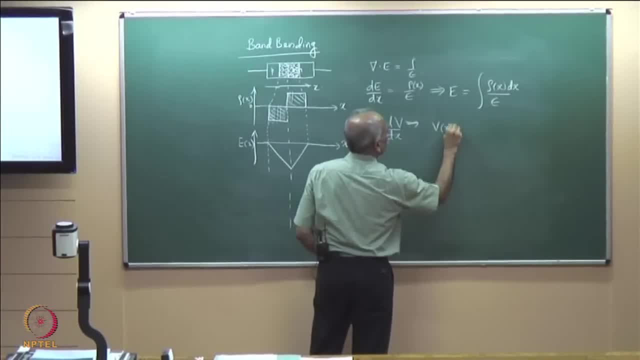 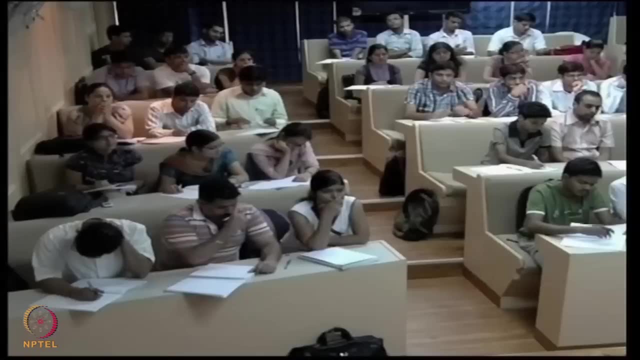 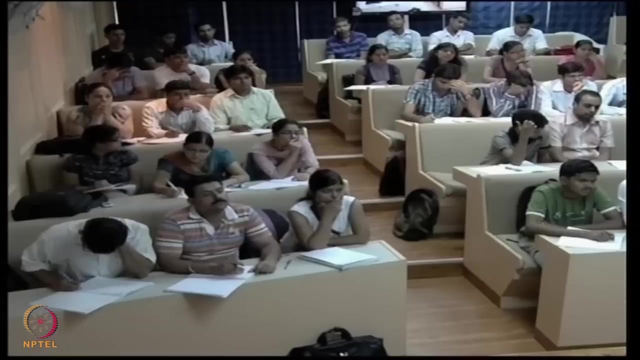 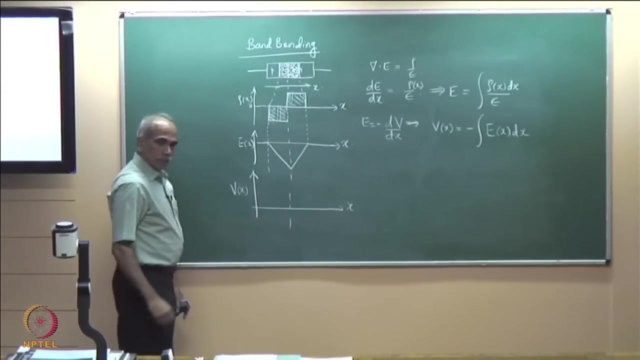 through d v by d x. Therefore, potential V, V of x is equal to minus integral E of x d x. V of x is equal to minus integral E x d x. So you further integrate. So now I want to plot V of x versus x. It is minus of E x d x. E x d x is integration. This is again. 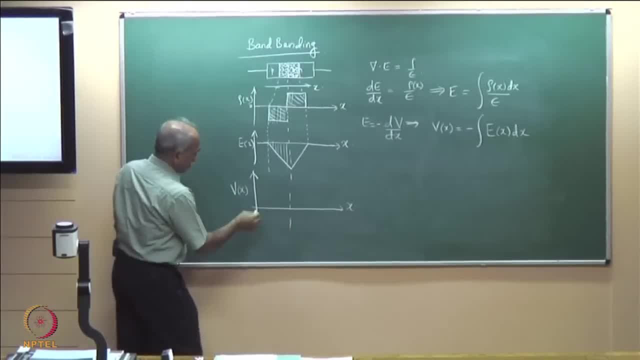 adding area here. So, but with a negative sign, therefore, this is already negative. With a negative sign, it is positive. Therefore, the potential starts from here and it starts getting increased. So potential increases like this: It increases till you reach up to a maximum. So this is what I 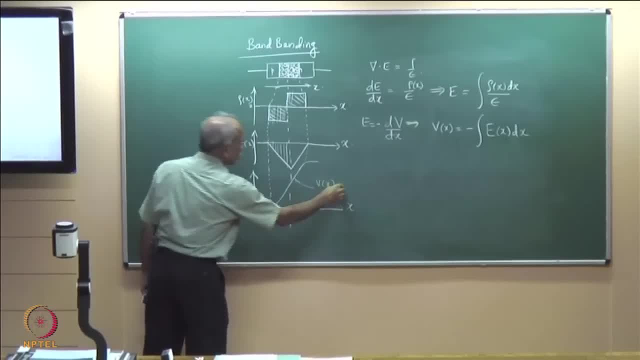 have plotted is V of x. V of x is simply minus e, x, d, x, integration. summing the area, just summing the area, and area does not get subtracted. Here it was negative, here it was positive. that is why it reduced and the field went like this. But now it is continuously going. 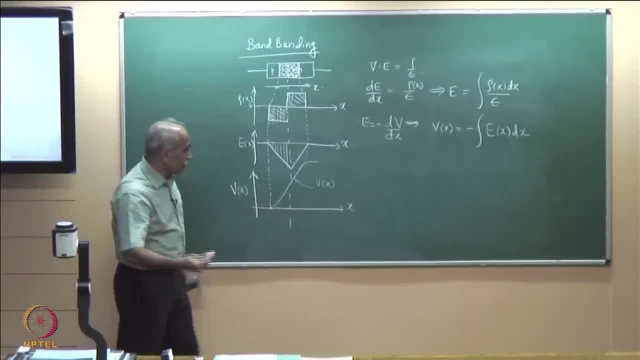 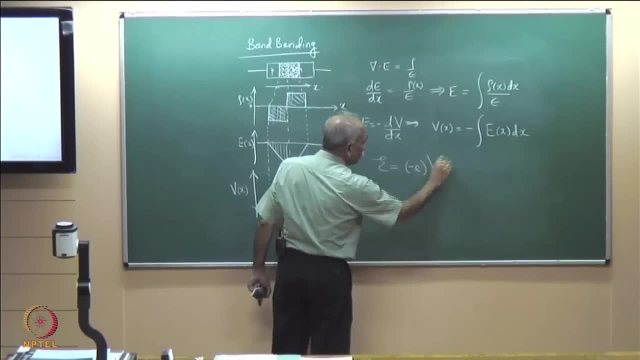 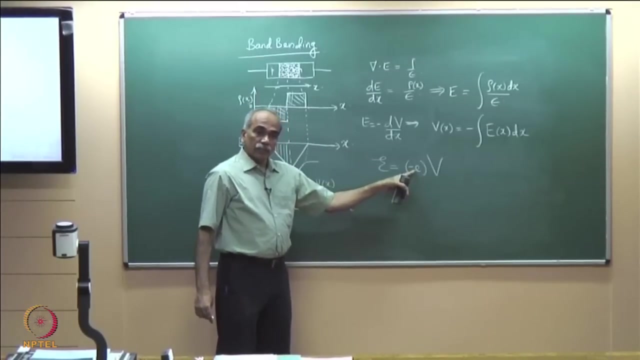 up to this. This is potential. What about potential energy? So potential energy: e is equal to q into V, that is, minus e into V. V is positive, e is negative for electrons. Therefore the potential energy. if I plot e, this e is not electric field. So this e is: 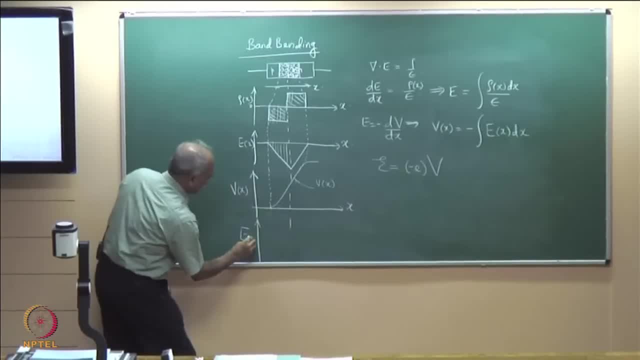 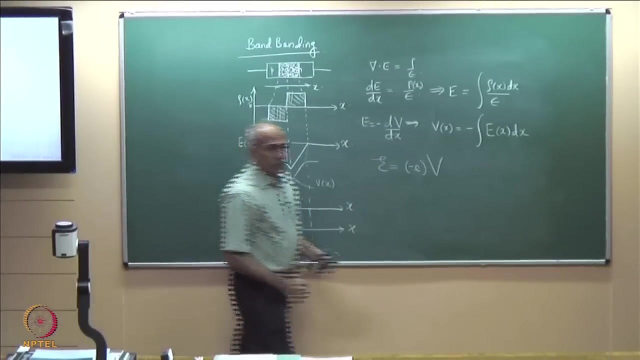 not electric field. This e is electric field and this is energy. Let me write energy. The corresponding potential energy is x, and So this is the potential energy variation across the general field. junction from 0 to some negative value because of charge migration. Because of charge migration. 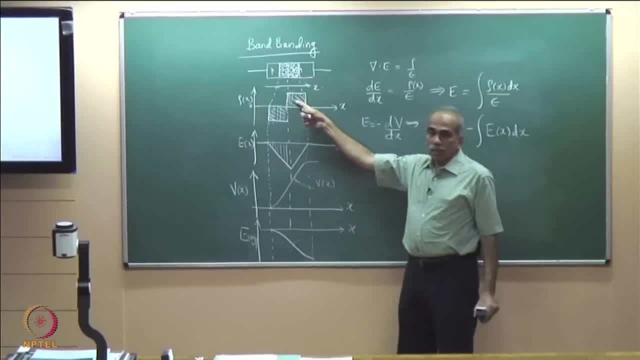 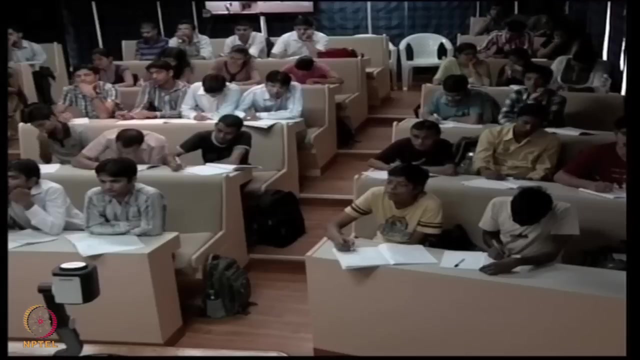 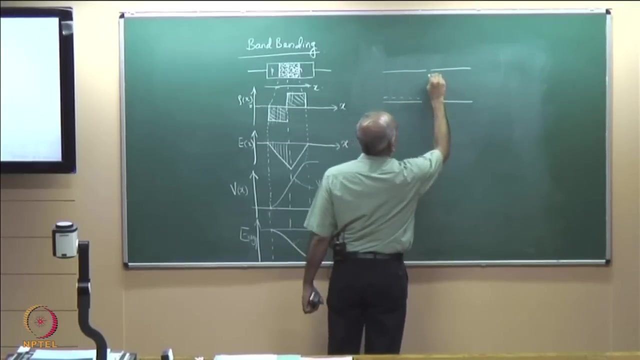 across the junction, we now have a potential energy variation. It is very simple now to realize the band diagram. I am sure you all know this. So this was the band diagram before contact. Now, because of charge migration from here and here, electrons migrating to 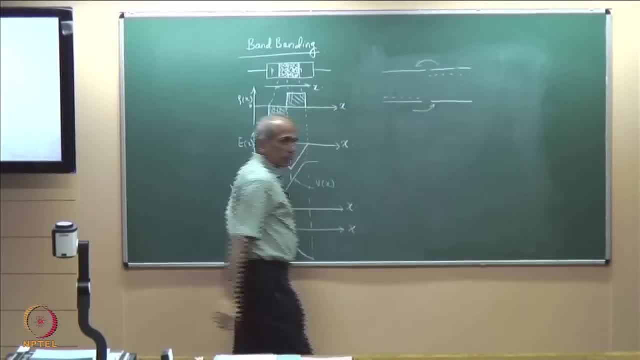 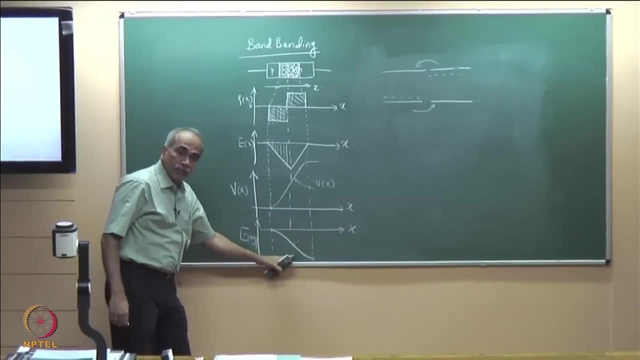 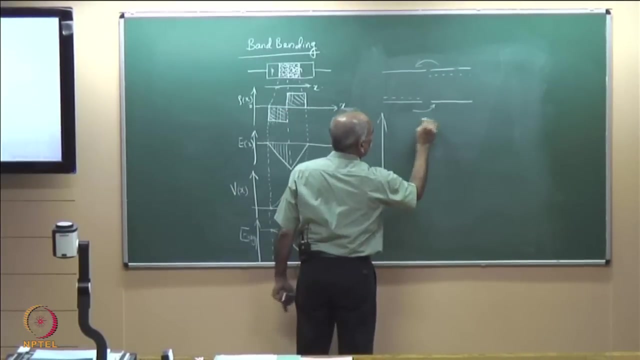 this side and holes migrating to other side. there is a built in potential and that corresponding potential energy variation is this: Therefore, now the total potential energy variation across the junction, This will be this plus a negative potential energy variation here across the junction. This is this axis is energy. The edges correspond to potential energy because kinetic energy 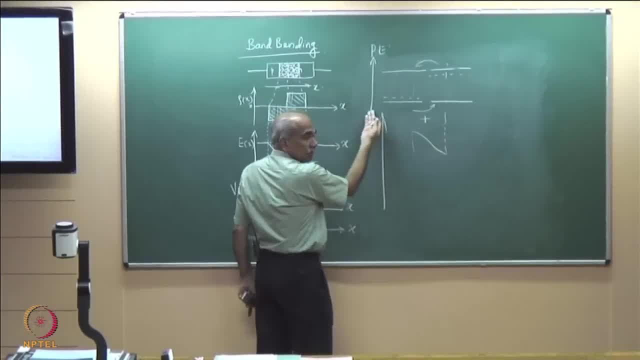 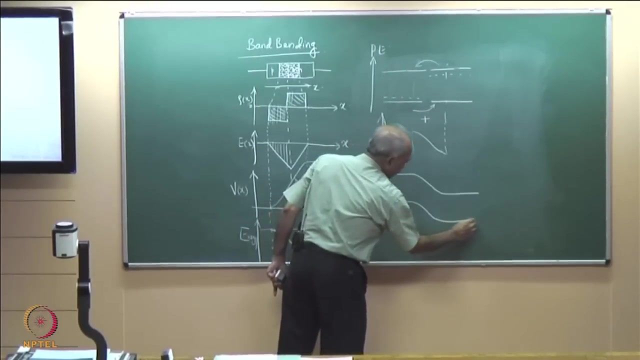 is 0 band edges, So this axis is energy plus there is an additional potential energy which is negative, And therefore, if you add 1 plus 1, that is this plus this. what you will get is the band diagram of a p n junction, And mathematics has already told us that Fermi level remains. 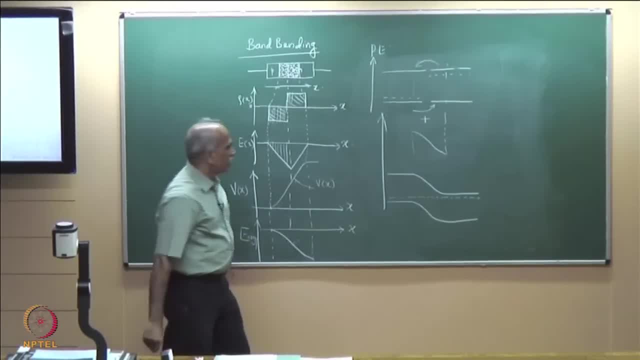 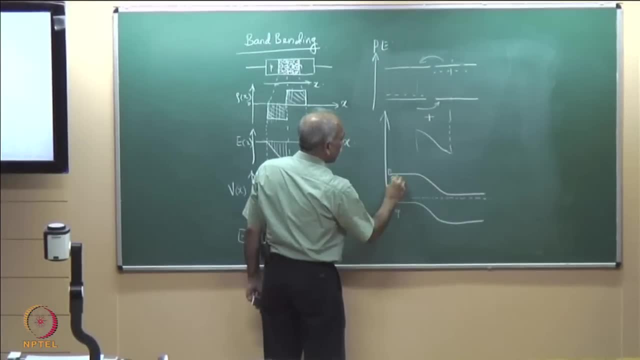 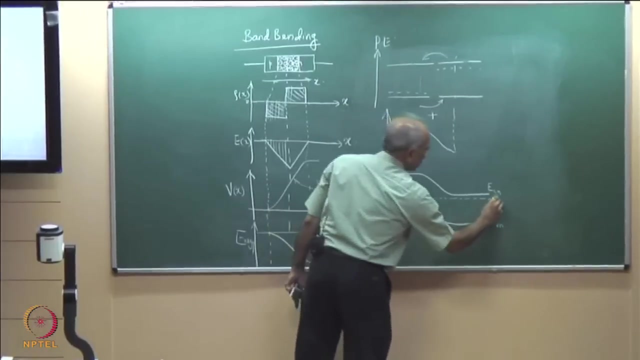 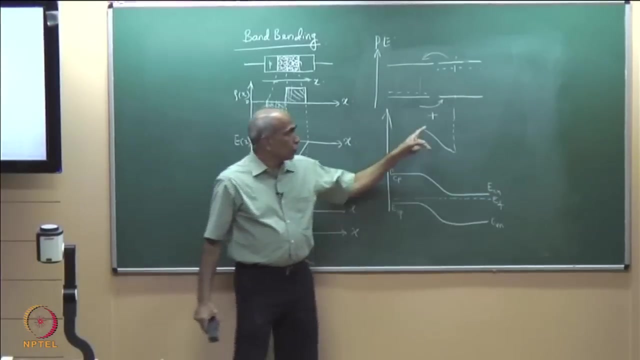 a constant. This is how we got the energy band diagram. So this is v? c, This is the e? v of the p side and this is e? c of the n side of, and this is the Fermi level. What I want, all of you knew this, but what I want you to see is only this point. This is very 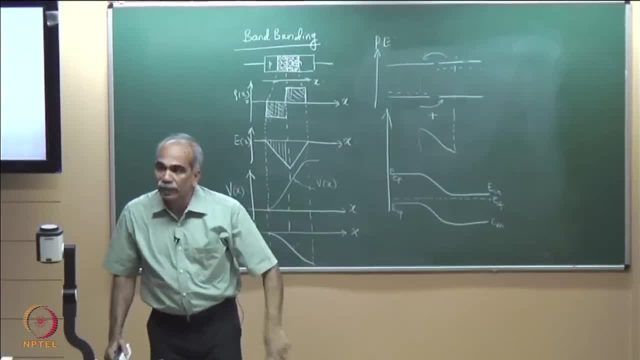 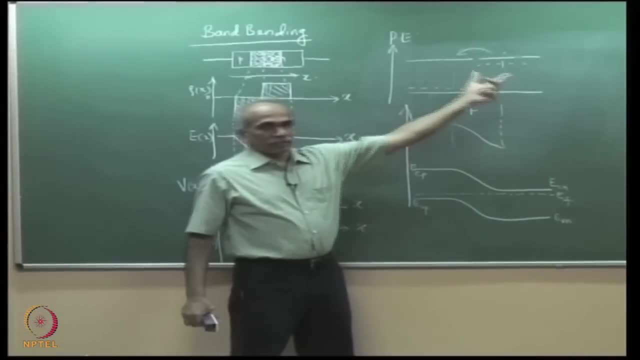 important now to see the p? n junction variation band diagram, to get the band diagram of a heterostructure That this has come because there was a potential energy variation. So this is the p? n junction variation like this: before charge migration and due to charge: 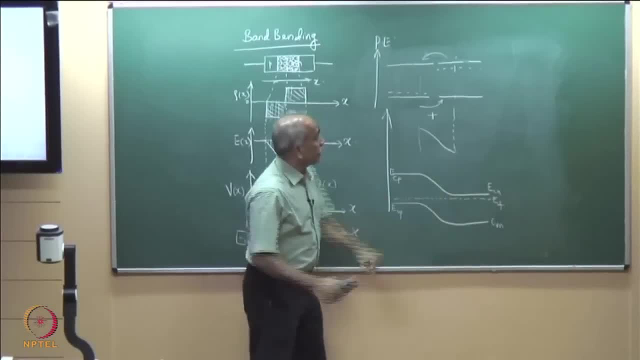 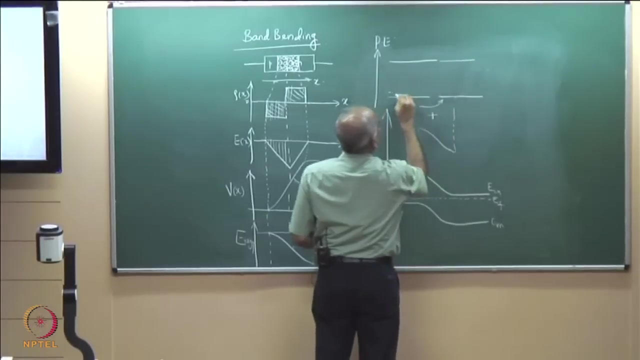 migration. there is a variation like this: Please see, if this side was p, what would happen? Let me erase this. This you have noted, So suppose. let me just make this side p. That is here I have n and this side is p. Now, electrons from here, electrons from this side. 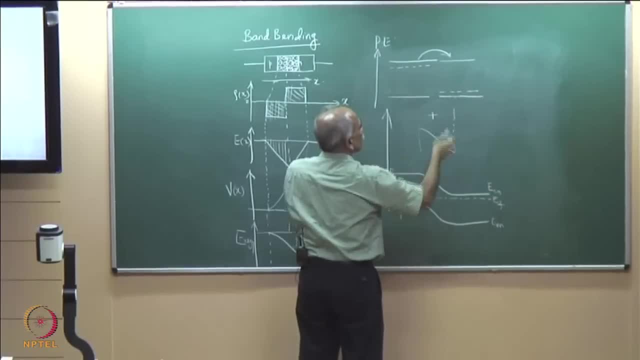 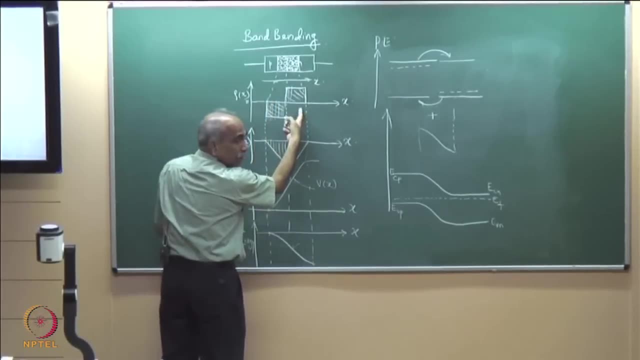 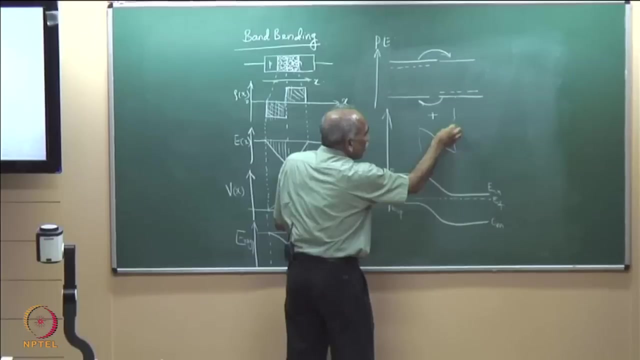 here would migrate here and holes from this side would migrate here. The charge distribution will reverse. That is this side you will have positive, this side you will have negative and therefore, when you integrate, you will get a potential energy variation not like this, but the inverse of this, That is, you will get a variation like this. So if you 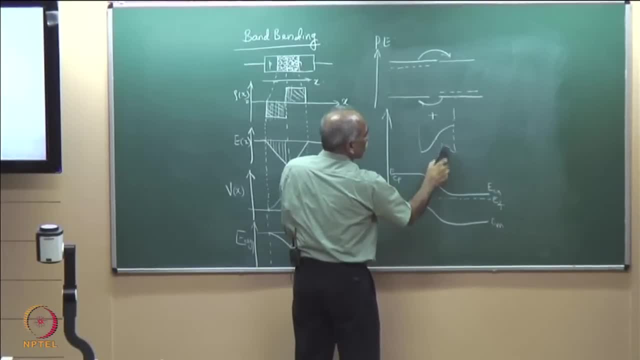 have p on the other side and n on this side, you will have a variation like this And correspondingly, the band diagram will be So we have the band diagram varying like this. So, given any junction, whether p- n or n? p or p? n heterostructure, we will see how to draw the band diagram energy. 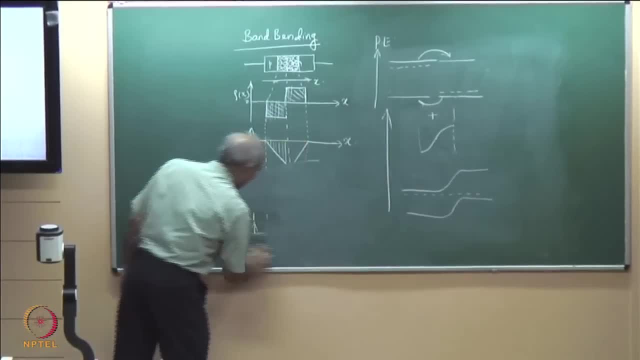 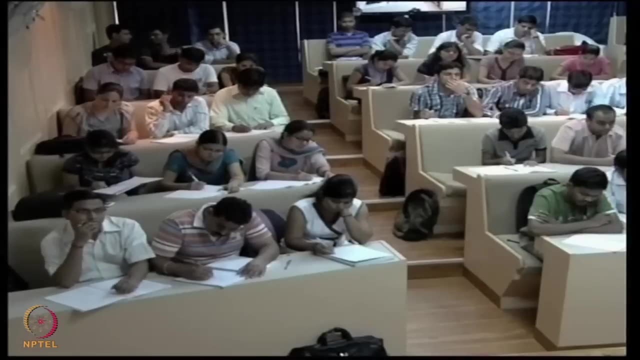 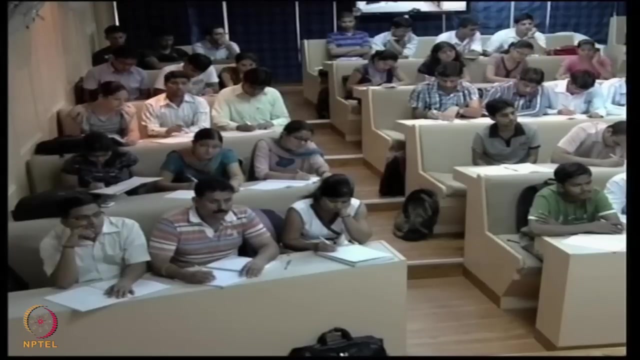 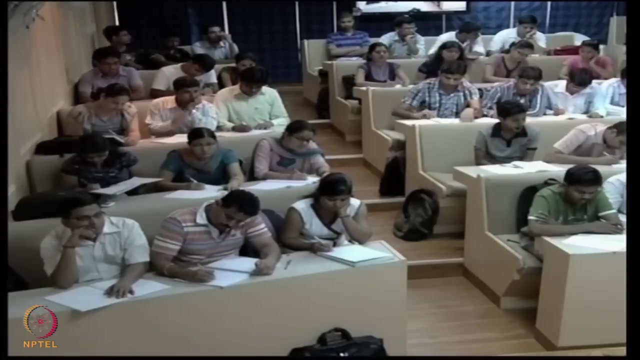 band diagram. This is important Because we will also see now that with in heterostructures we have band gap discontinuities and this makes a difference, because when you have p? i? n structures or p? n- p structures, then there are potential barriers and potential wells which confine or which block the flow. 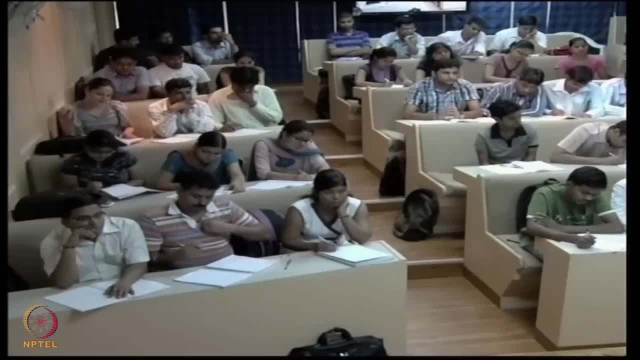 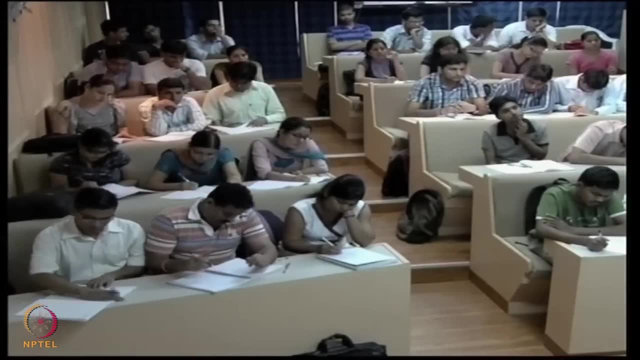 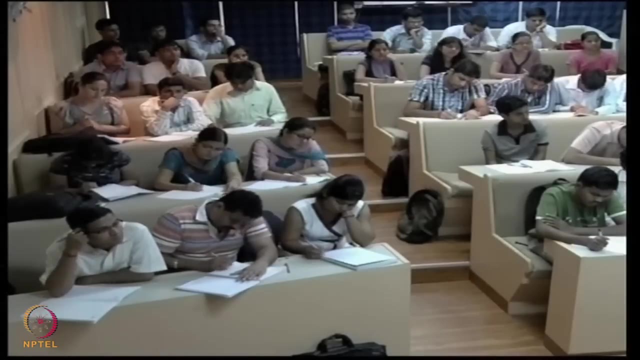 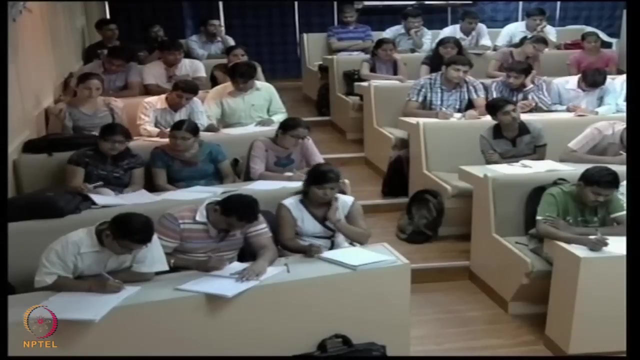 of carriers And they have performed Importance in the characteristics of the device. So let me take now p? n junction of a heterostructure, A single heterostructure that is not double heterostructure. First let us see the p? n. 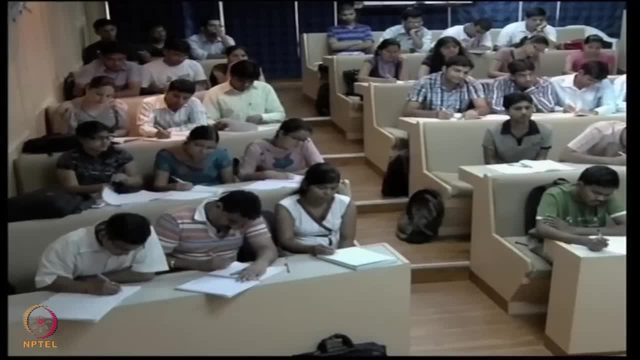 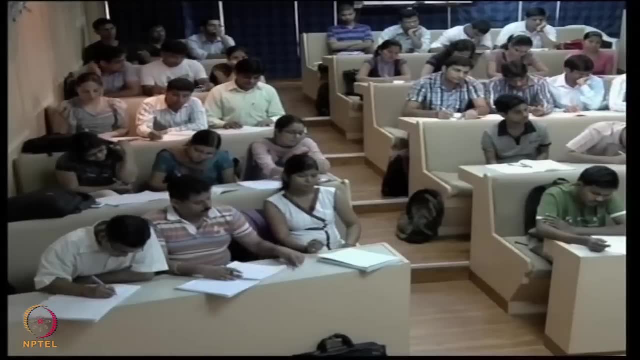 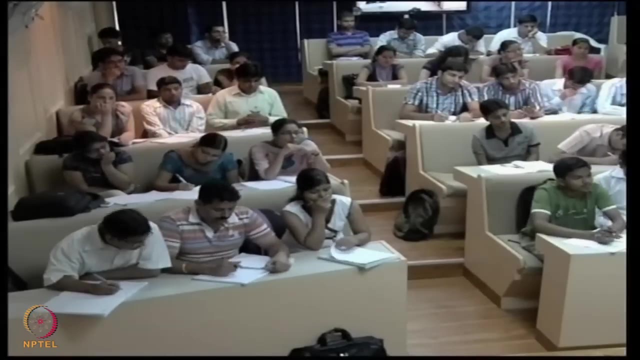 junction corresponding to a heterojunction, and then we will see a double heterojunction And the potential barriers and wells which are created there are very important and crucial to the performance of the device. So let me take aluminum, gallium, arsenide. Let us say 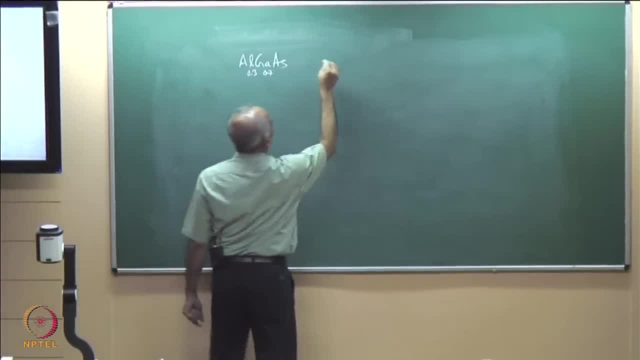 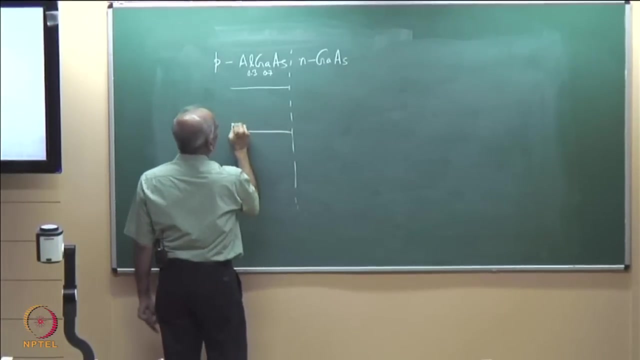 Al 0.3 gallium, 0.7 arsenic and gallium arsenide. Let me take this as p type junction between a, p, n. so here we are. So you have p type gallium arsenide, n type, and we know that there is discontinuity, approximately 65 percent, and 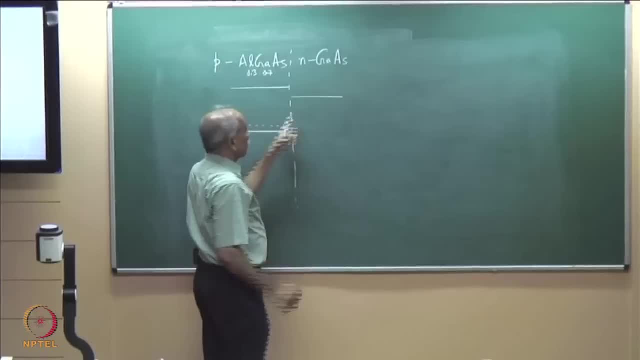 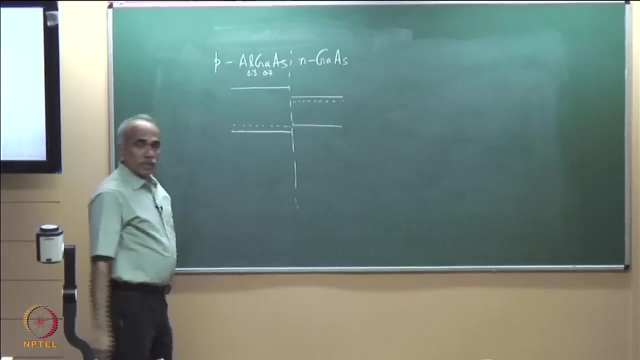 35 percent. This is the discontinuity which is considered to be the discontinuity of the hydro gel: 0.6, 0.6, 0.6. So this is n type gallium arsenide, If you take intrinsic material of aluminum gallium. 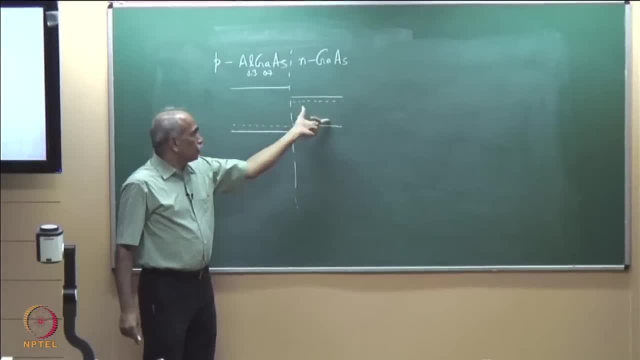 arsenide and gallium arsenide and there is no difference in the carrier concentrations, then we have 35 and 60, 65 and 35 the difference. If you have carrier concentration difference, then there is flow of carriers and we will immediately have, in addition, a band gap variation. 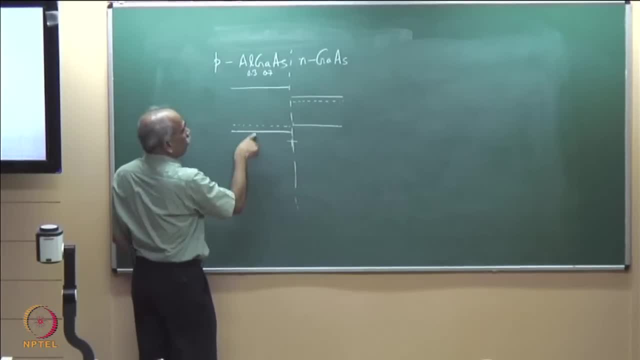 a potential energy variation. That is, this is p type now and this is n type and therefore there are large number of electrons here and large number of holes here. So you can see very large number of holes and there are very few holes here and immediately when you make 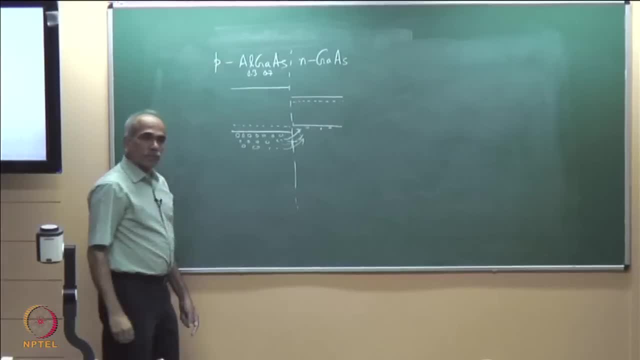 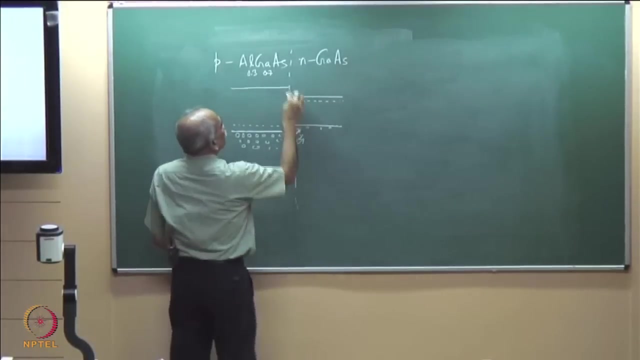 contact, This will immediately start going to the other side. The air bubbles are moving to this region, So when holes move to this side, this becomes So what you have here, So you will be left with negatively charged, negatively charged, immobile ions. Let me show in the 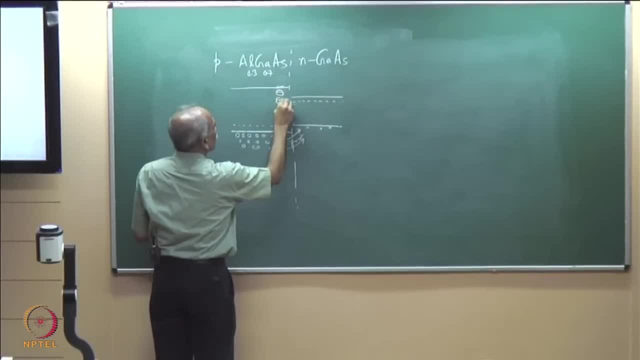 band gap itself. So because of hole movement, or it means electrons are coming from here to here, Hole is moving that side because electrons are coming this side. One additional electron makes the immobile ion negative. That is why you have negatively charged immobile ions. So when this end becomes, 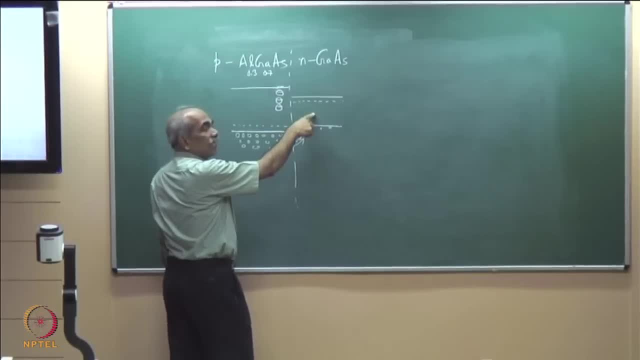 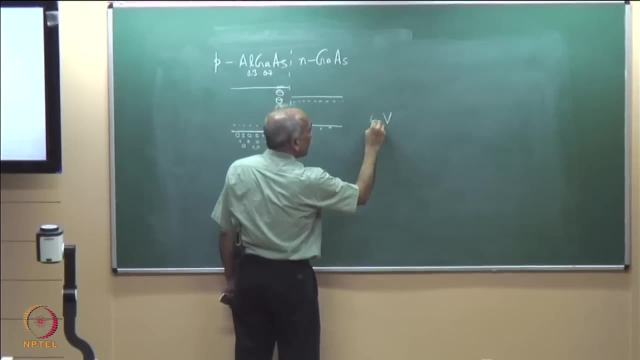 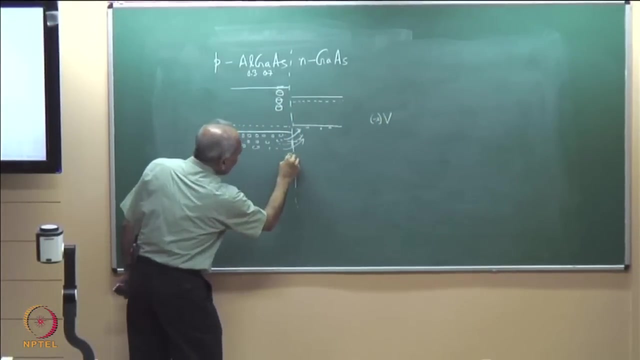 more positive. compared to this end, the potential energy decreases. more positive. Please pay attention. Please see: V is positive but multiplied by minus E is a negative quantity. Therefore, this end decreases and that is why, if you want to find the net band diagram, then we. 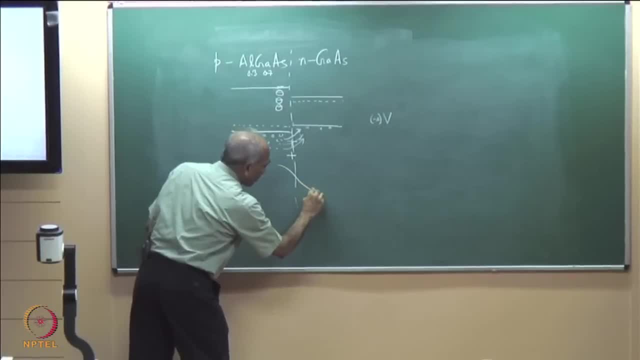 have a potential energy variation because of carrier migration. This is the potential energy variation because of carrier migration- Just know that we have seen this- plus a band band gap variation. So if we plot the sum of these two, please see, So we have variation which is coming. 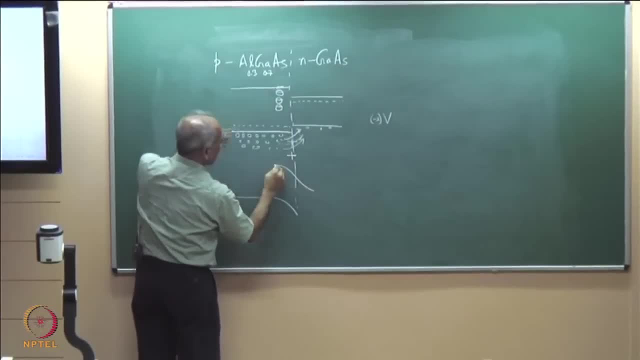 like this. So it has come this minus this. This is zero, this level is zero and there is a negative, So negative is added. Therefore, this is going down. but when it has come to the junction, there is a delta E- c, There is a discontinuity of the line. So this is: 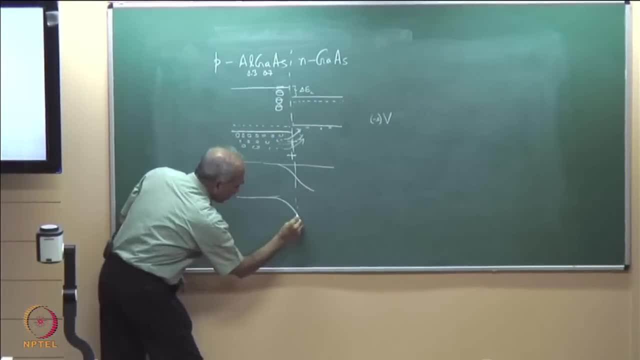 here, which is downward discontinuity, which means- I have come up to this- and there is a downward discontinuity of delta E c because it is a heterojunction, this minus this. So the band was bending like this. So when it has come up to the junction, there is a downward 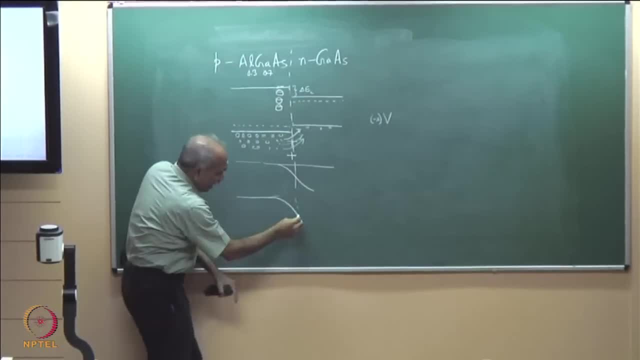 discontinuity because of a heterojunction, So the same downward discontinuity will be shown here, and then you continue with this, So this continues and finally, so this is the upper one- E, c, I have shown this line only. So this plus this, keep on adding this. 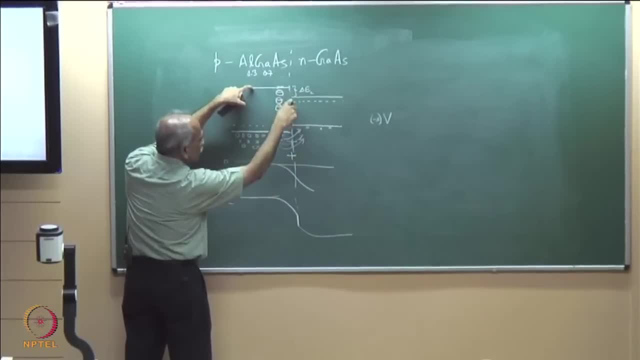 plus this: you come up to this: there is a downward discontinuity, and then again keep on adding. So this will go like this. If the discontinuity were not there, then it was like our original p? n junction. this would have gone like this: 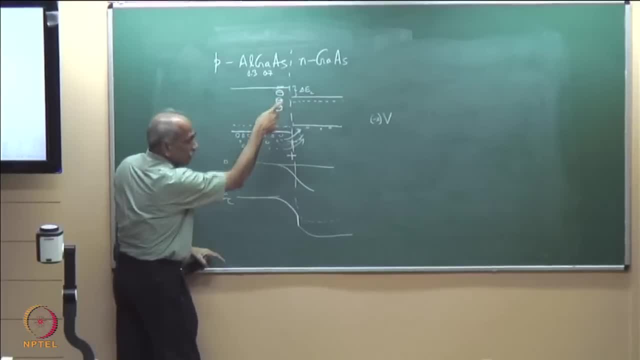 But because of this additional discontinuity, we have a discontinuity shown in this band, upper band. Let me draw the lower one. it will become clear once the picture is So same gap, I keep the same gap, So this starts bending. it comes up to this, So it is bending. What? 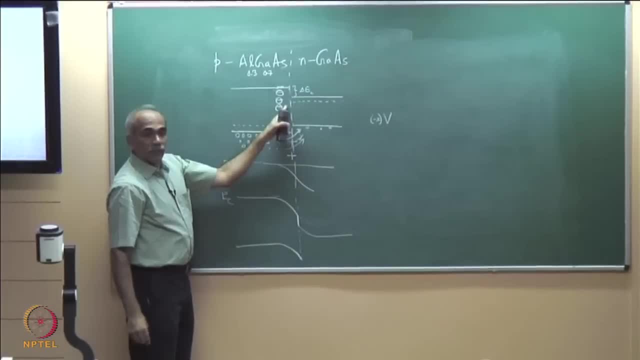 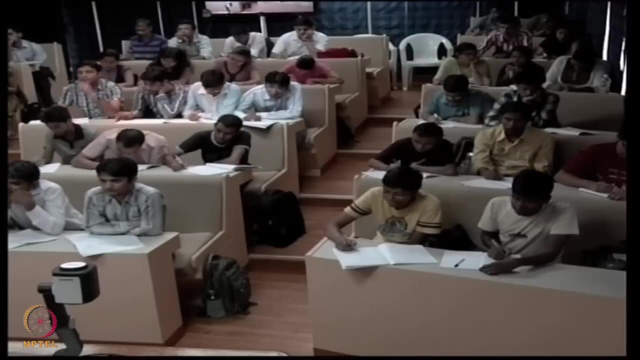 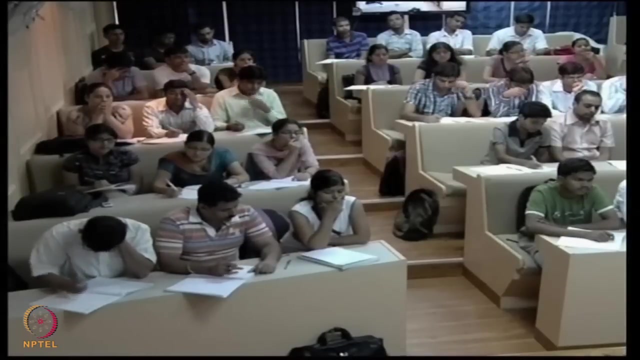 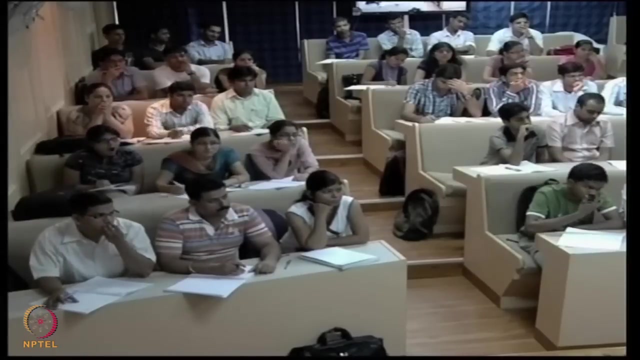 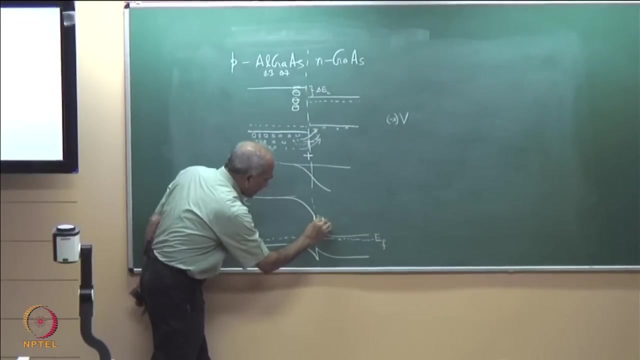 will happen. at this point There is an upward discontinuity, So the band has an upward discontinuity and then it continues and the Fermi level must remain the same. Yes, this discontinuity here is the same as delta E c which we had here, and there is a. 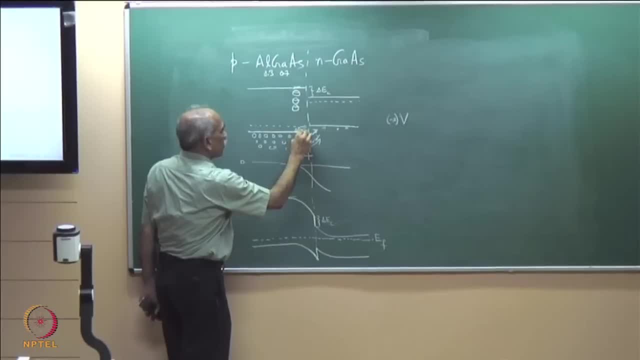 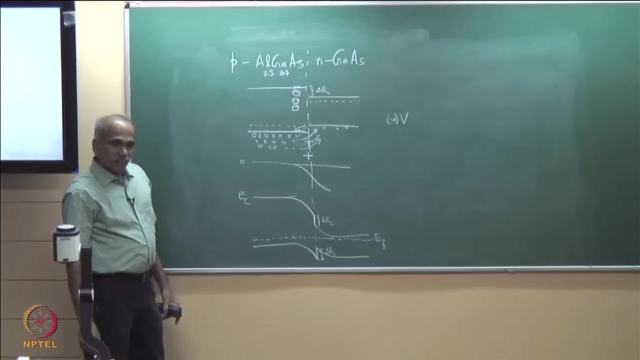 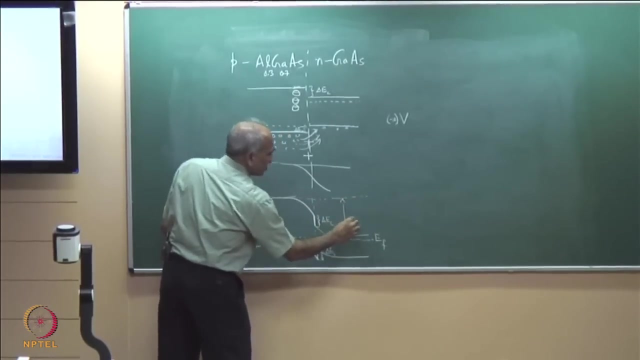 delta E v here and this discontinuity here is delta E v, So the band diagram looks like this. So what has happened? So what has happened? So what has happened is one: the built in potential is much larger now. This is the. 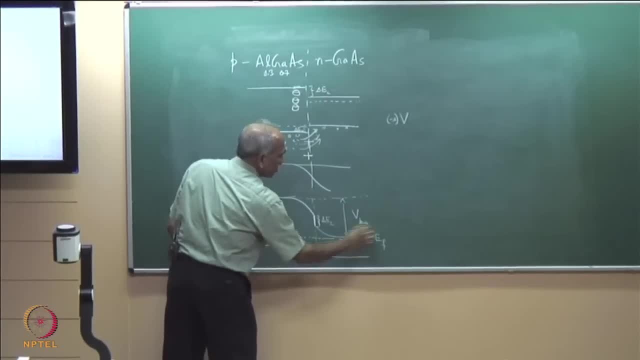 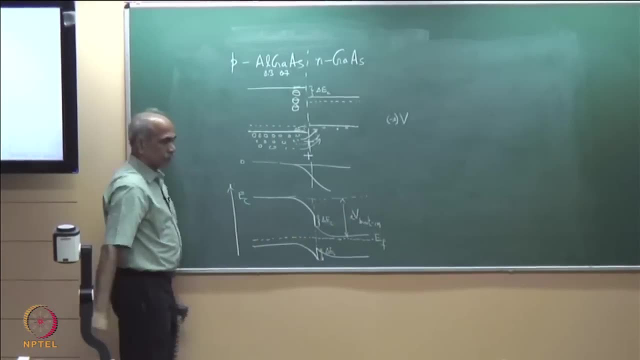 built in potential V built in or E times. if it is energy axis E times V built in, Some people just call it as built in potential V, sometimes because of energy axis E times V built in In a heterostructure, you can see that the net barrier height has become much. 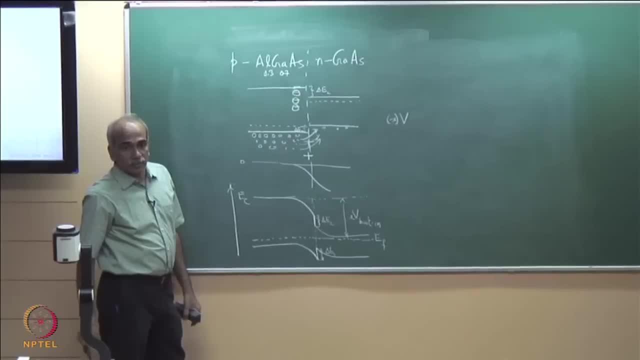 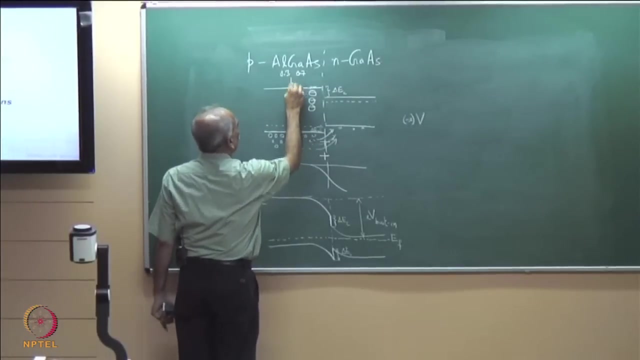 larger. The built in potential is much larger. You can practice with any types of any different types of any type of heterostructure, hetero junction, a single hetero junction. What I have done is for P? n, you can do for N? p. you can also have this smaller and this bigger. 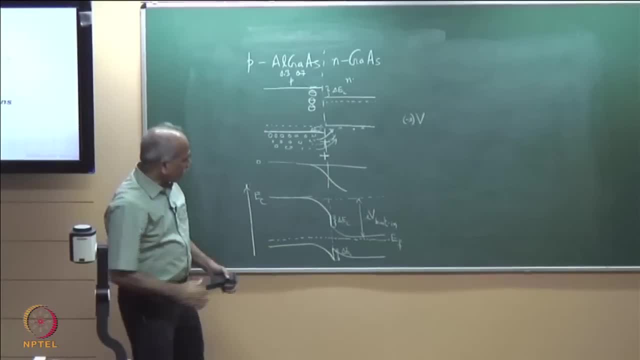 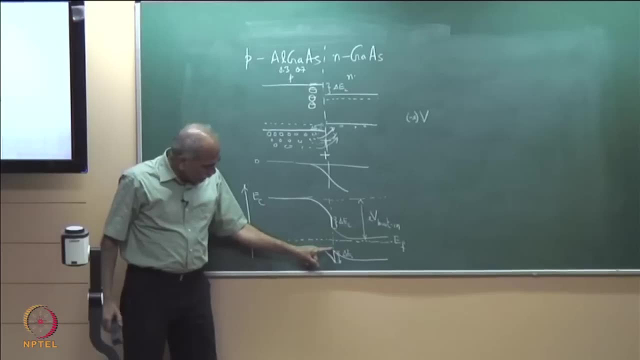 So see what kind of band diagrams you get, Just to practice that, yes, you are able to draw this p? n junction. So the discontinuities band gap discontinuities will now appear at the junction. The most important thing that we need is what will happen in a double heterostructure. 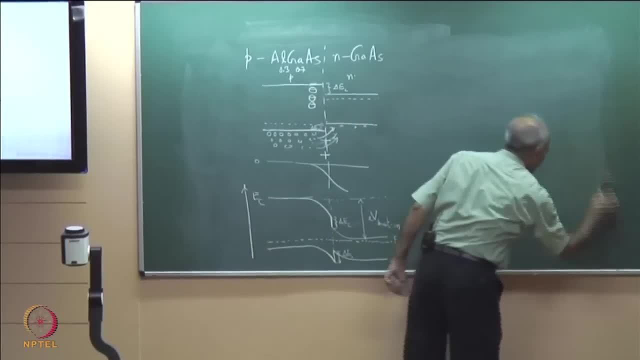 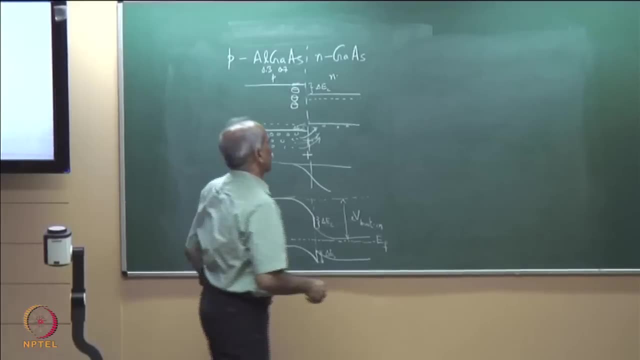 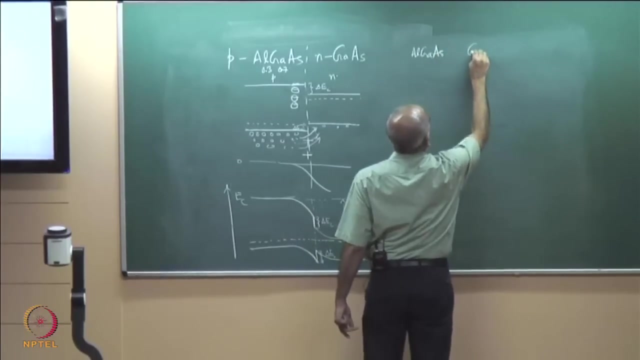 We will encounter this later in a laser, but let me draw the band gap of a band gap, variation of a double heterostructure. So again, let me take: So we have the aluminum gallium- arsenide, gallium arsenide and aluminum gallium- arsenide. 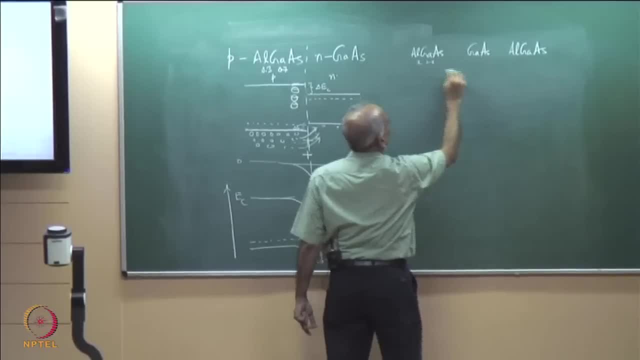 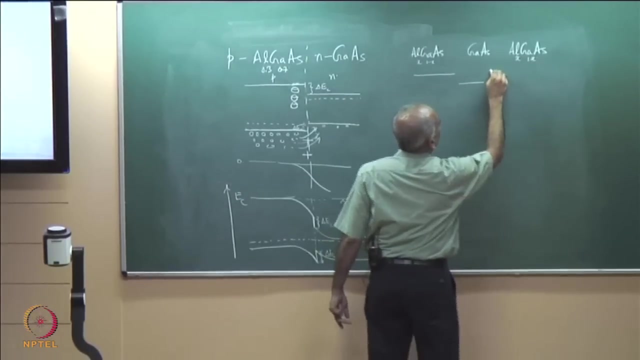 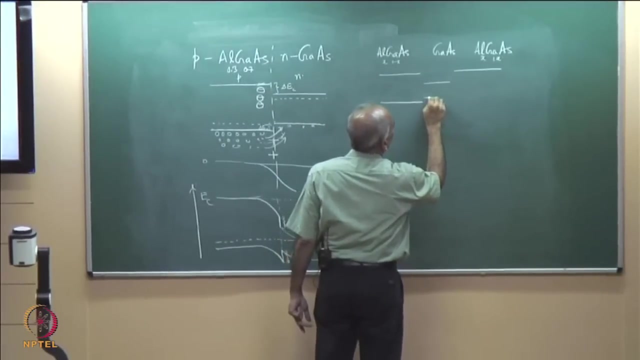 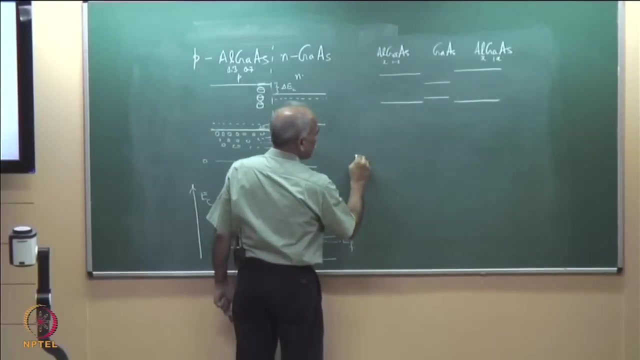 You can have any composition: x 1 minus x A s, x 1 minus x A s- same composition or something different. it is possible to have different compositions also. So we have this and we have Sometimes. you may also have materials where the upper layers are aligned. one of them may: 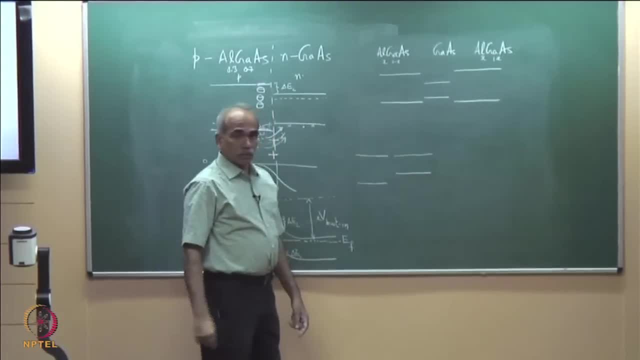 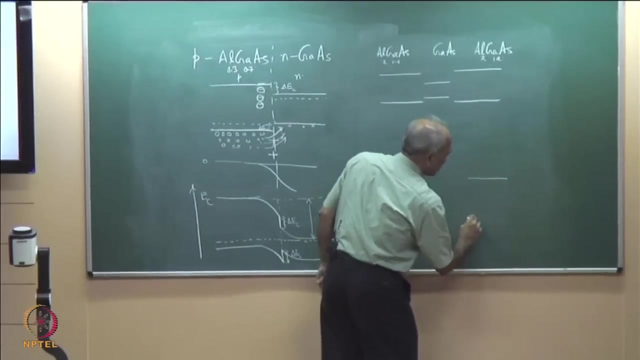 be like this and another may be like this. It depends on the material and the electron affinity. Electron affinity of aluminum arsenide is much smaller compared to that of gallium arsenide. You know what is electron affinity? Electron affinity is the amount of energy required. if this is E c and if this is E v. 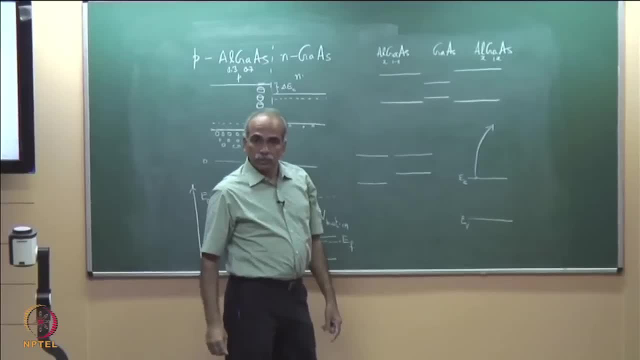 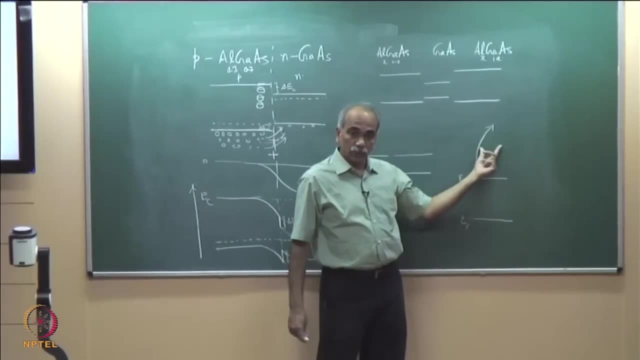 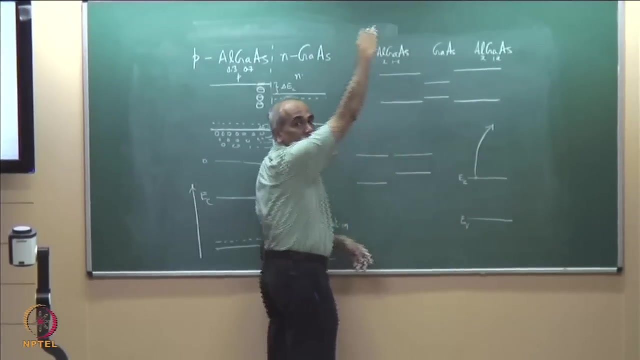 amount of energy required to free it. So in the case of aluminum arsenide it is approximately 2.2 or 2.3 electron volts, whereas in the case of gallium arsenide it is about 4 electron volts. That is why you see gallium arsenide is sitting below aluminum arsenide is up. 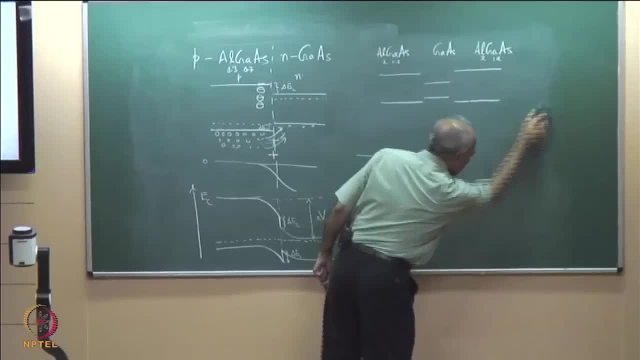 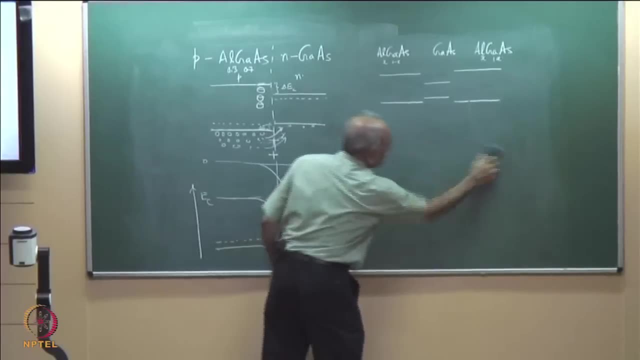 More details you can refer to books, but let me draw the band diagram corresponding to this, because this is the kind of structure which we will encounter. This is a double hetero structure, which means a low band gap material is sandwiched between two high band gap materials. 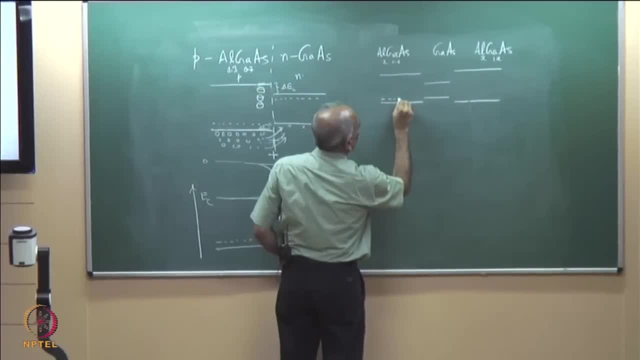 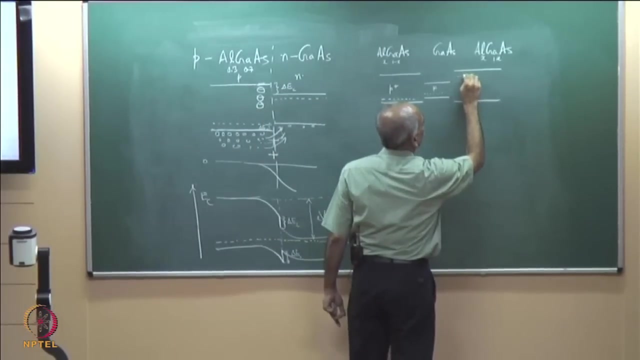 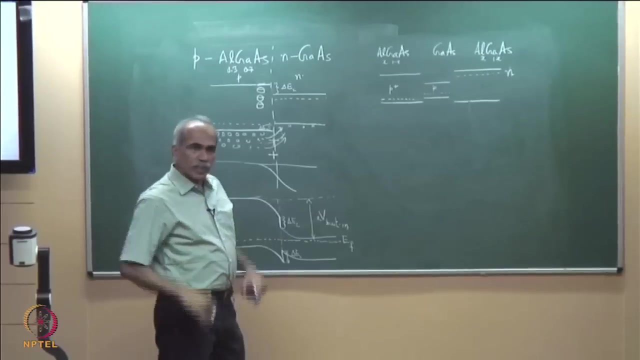 So this is a p type. I have p type here. This may be. let us say so. this is p plus. this is slightly doped p. It could be intrinsic as well, and this is n type. N, This is n type. Try yourself how the band diagram should vary. 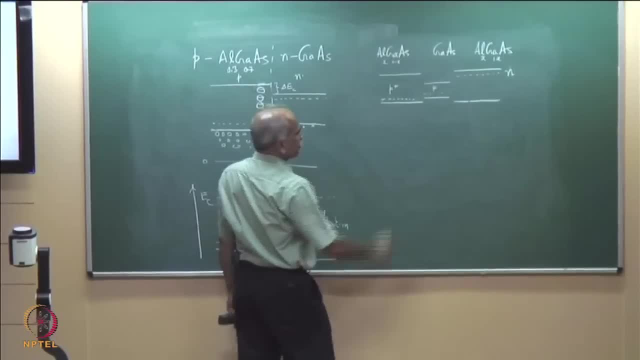 So there is a delta E c, delta E v, So at every junction. so this is like p? n. so we have a variation which is like this: So, plus this potential energy variation because of charge migration, This is also a p? n type of variation. 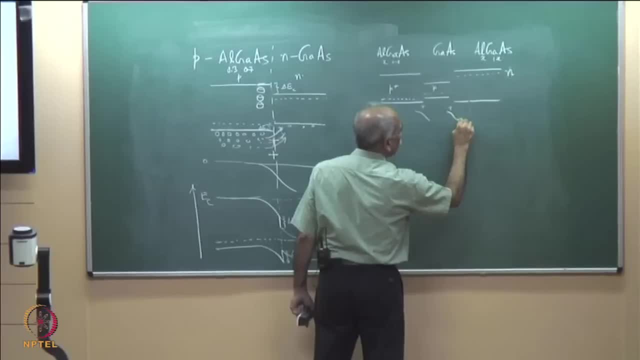 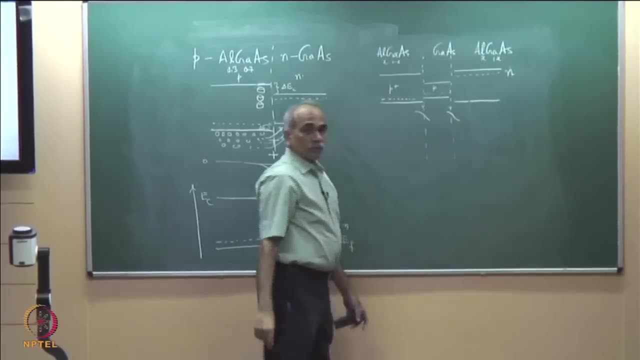 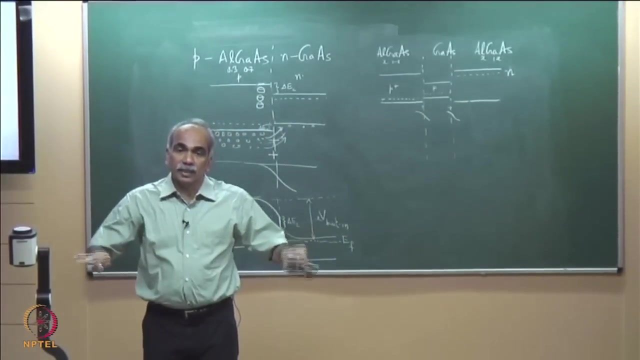 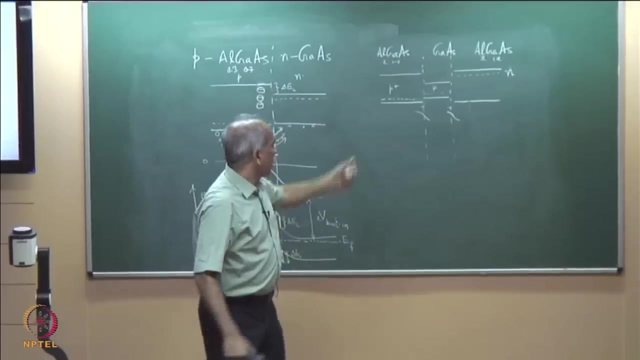 Therefore I will have an plus at this junction also, we will have a potential energy variation. And the last point is: Fermi level should become constant When you make the final junction. p plus p? n. this is the typical structure of a double hetero structure laser. we will see later that we have to draw the band diagram. 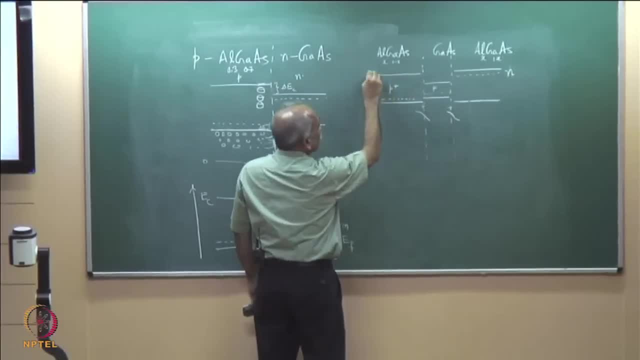 Let us start- I am drawing this the upper one, E c. so E c continues. it is reaching here, therefore it should start bending now. it bends exactly the band as it is, and then there is a discontinuity: downward discontinuity. delta E c: downward discontinuity. please see, this is the delta. 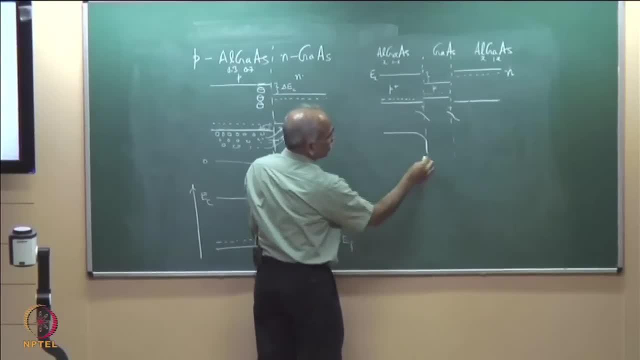 E, c, downward discontinuity. So I have a downward discontinuity And then this continues like this and then it is flat. so it is flat. Now I meet the second junction here and therefore there is a second potential energy variation. so this starts bending again like this. 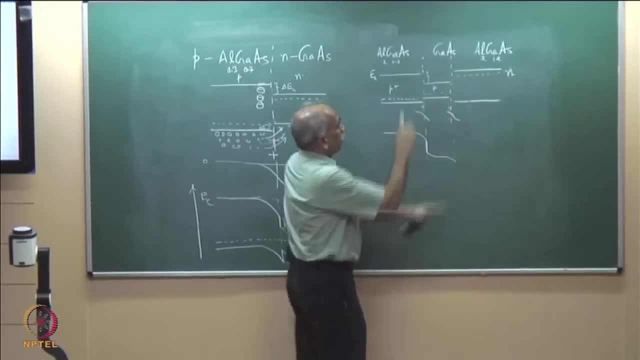 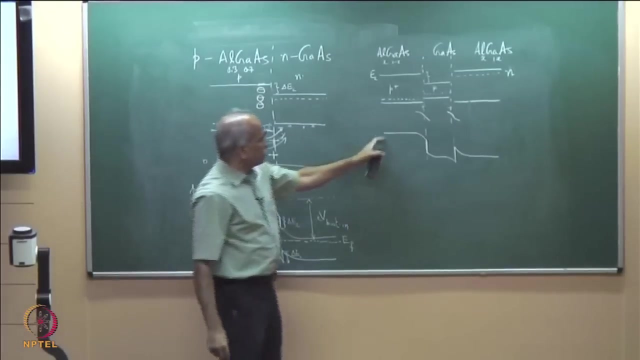 At this point. it has come here, so this is where I am. please see, I have passed this. I have come here. now There is an upward discontinuity, so upward discontinuity because of this, and then this continues. This is only the upper line, exactly like this. the lower part. 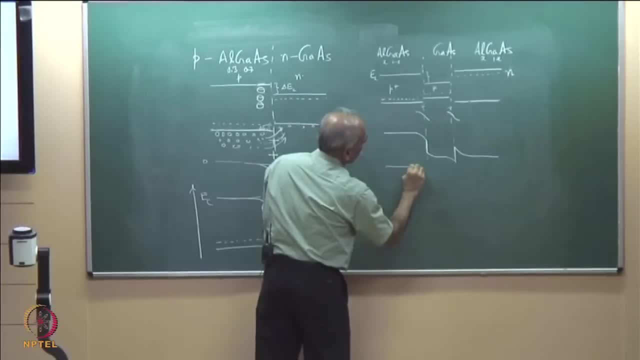 So keep the same line, Same separation. do not worry about fermi level. let it come wherever it comes. it bends. here the discontinuity is upward, so I have an upward discontinuity, Then I continue further. I come here, there is a downward discontinuity, and then I have 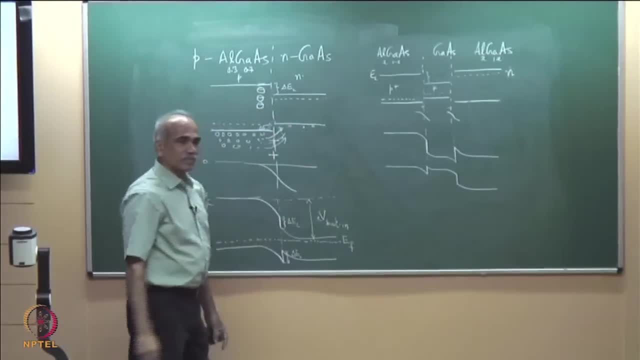 this. So this is a downward discontinuity, So I have an upward discontinuity. Then I continue further. I come here And there is an upward discontinuity. So I have an upward discontinuity, So I have a downward discontinuity. 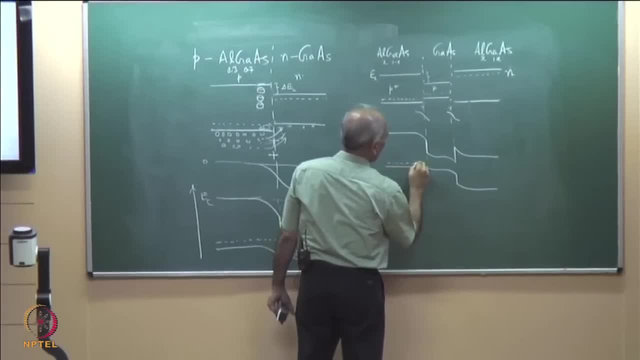 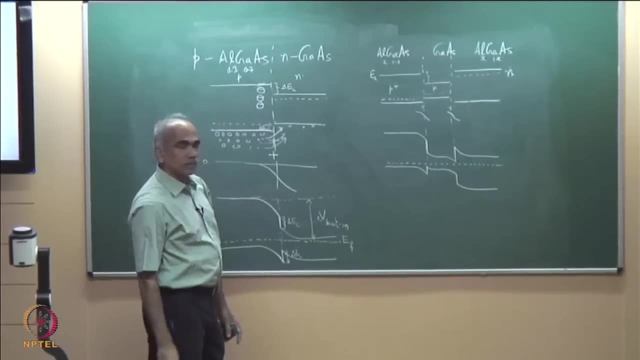 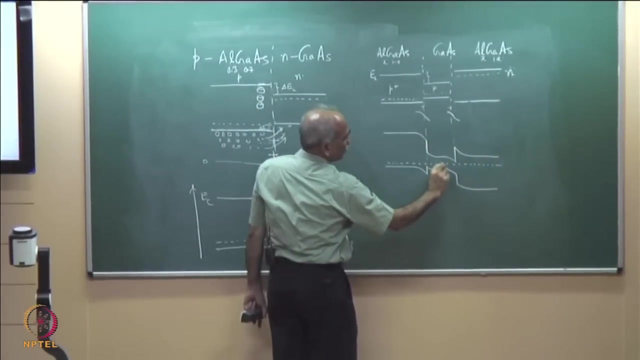 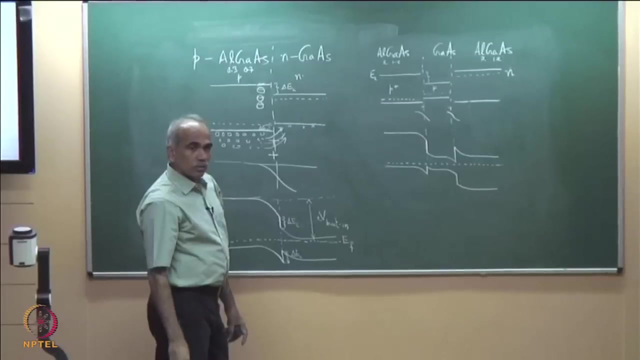 Then I continue further. So I have an upward discontinuity. So fermi level is constant and you can see that this is n here. this is about a little bit p, slightly p doped, and this is highly p doped. what do you see in the structure? compare: 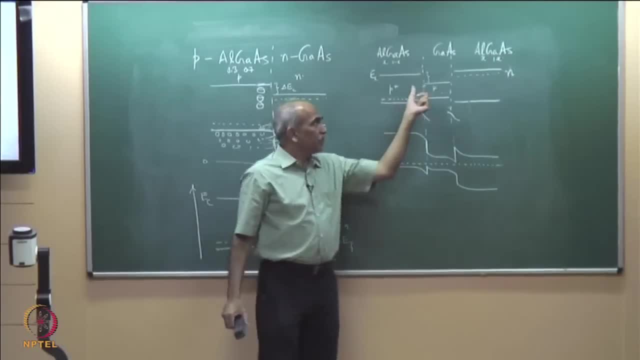 to a normal single homo junction. what do you see in a double hetero structure? That in the, in that intermediate layer, which is going to be our active region, that you have a potential. well, you have a potential well here, and we already had a potential well. 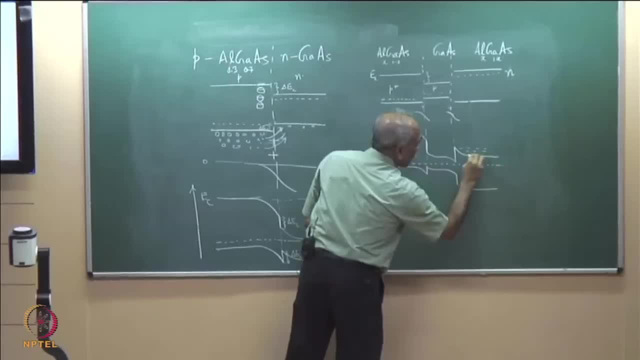 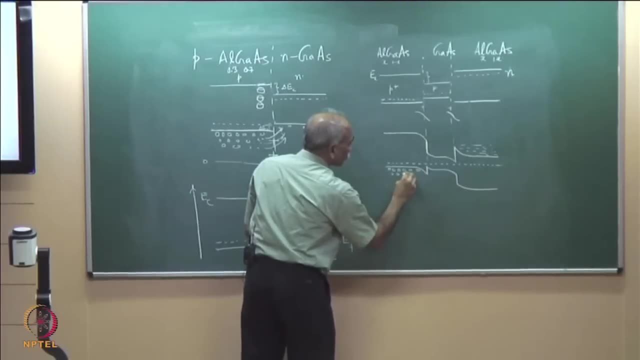 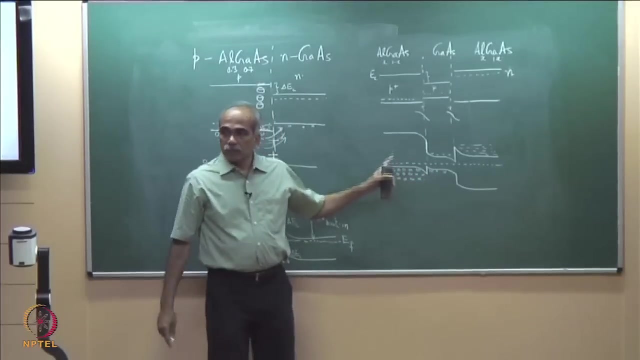 but there is a barrier. So here you have full of electrons, here you have large number of holes. some holes have migrated here and some electron has come here. So this is under no bias. it is a double hetero structure. band diagram of a double hetero structure. this 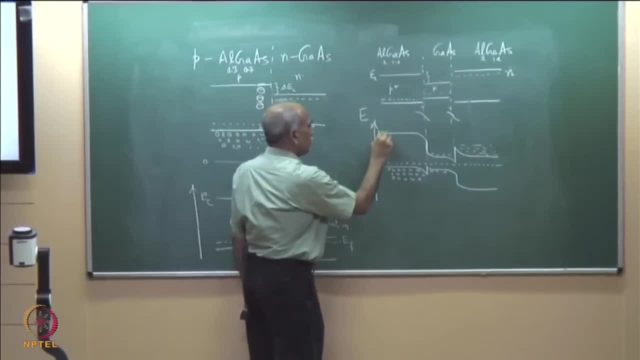 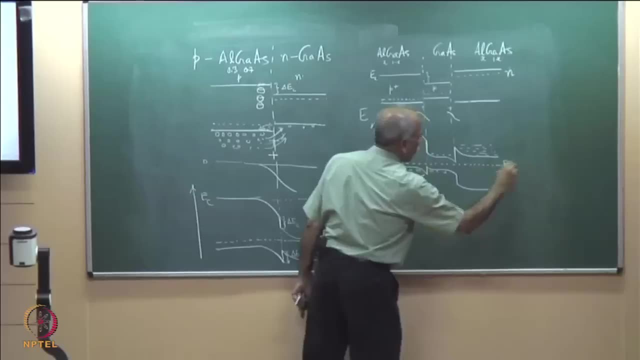 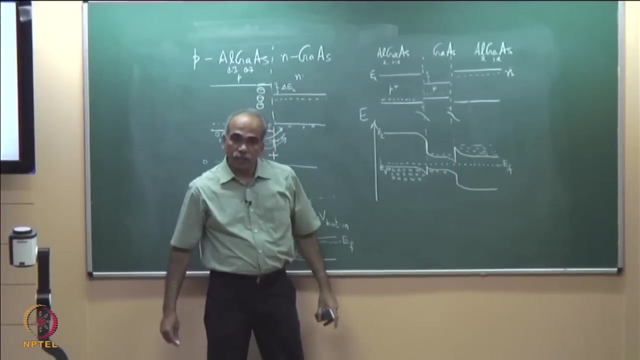 is E, This is E, c, E, v and this is E, f throughout. this is of the p side and similarly, E c of the n side, E v of the n side, and this is the intermediate region. Let us see what happens. 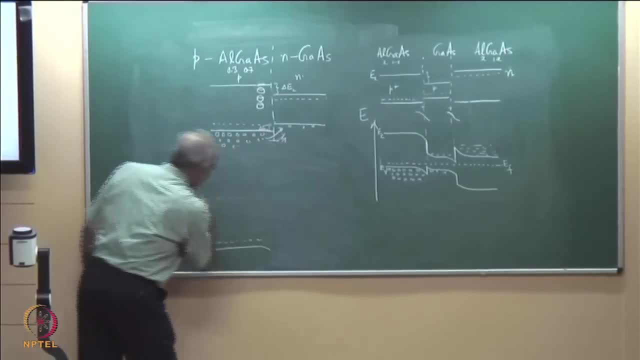 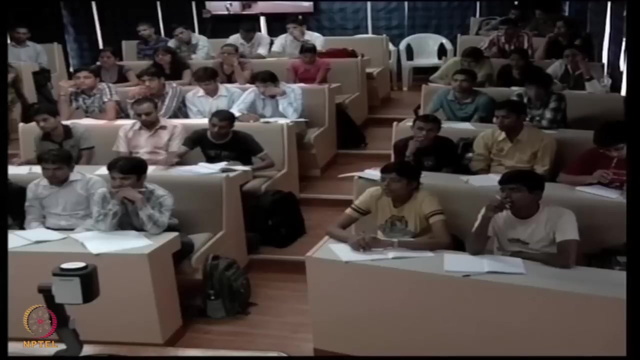 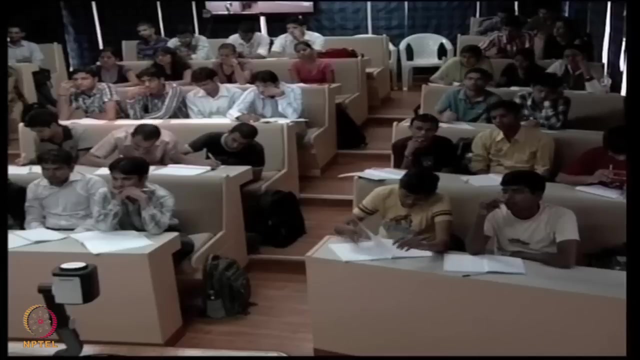 Why am I interested in double hetero structures? Once we know this, then rest of the physics will follow. when we discuss 1, the laser diodes, we do not have to again come back to band diagram. we know, yes, this is what happens. This had a major implications which led to the CW operation of laser diodes. 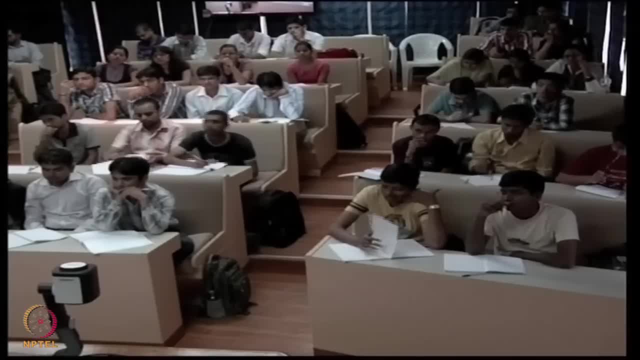 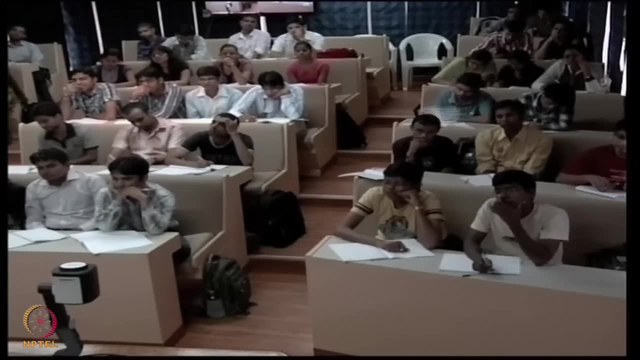 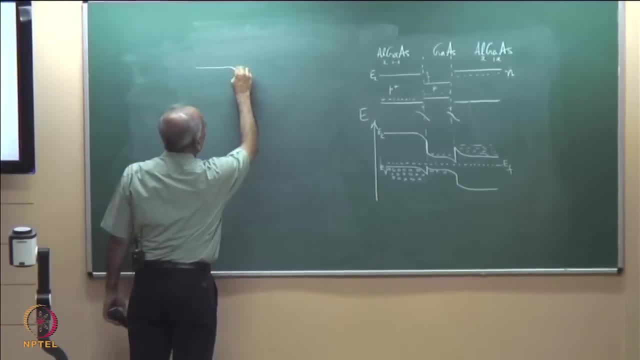 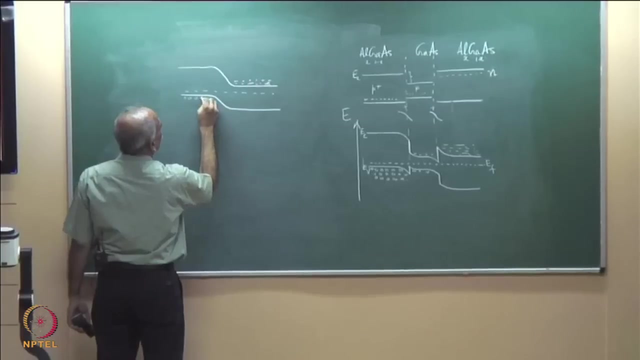 and subsequently, after many years, recognized as one of the finest discoveries and noble prize was given. See such a simple idea if we take a homo junction. if we take a homo junction, there are large number of electrons here and large number of holes here. This 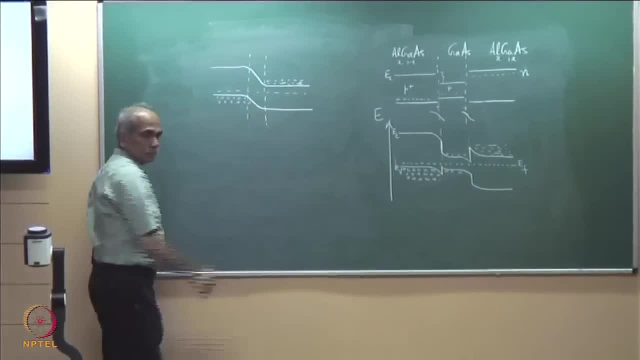 is the junction, The junction region or the active region, so this is the p type and this is the n type. There are very little electrons and holes in this, so this is x special coordinate. There are very little holes or very little electrons in this region, which that is why. 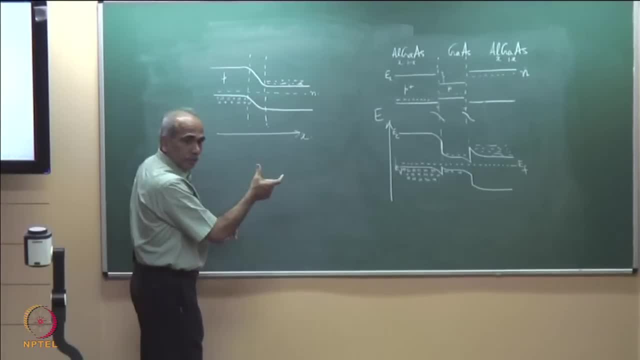 we called it as a depletion region. If you forward bias this, which means you are applying positive to this side And negative to this side, What would happen? This band would go up. Why would it go up? Because electrons are getting additional negative potential. It is negative, but the potential 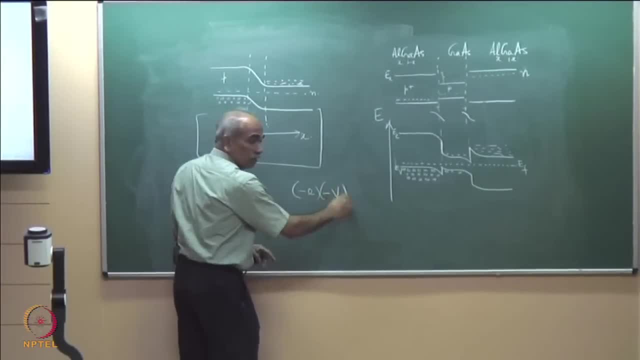 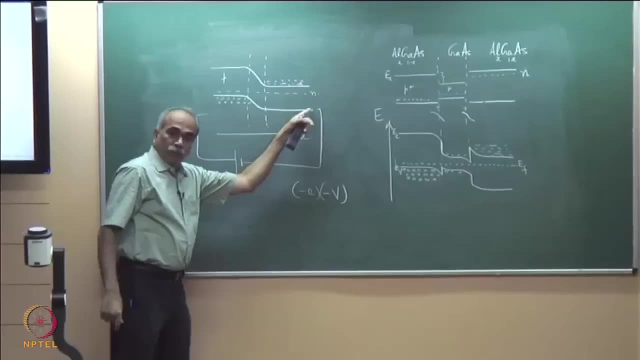 energy becomes minus e into minus v is positive and therefore that is why this band goes up. As you apply a forward bias, this end starts going up. So when this end starts going up, this band goes up In the same region. let me draw in the same diagram. I hope you can. 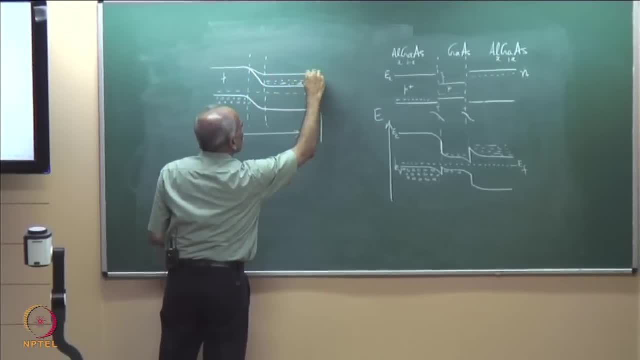 recognize it. So this has come up here and correspondingly, this has come up here. This is with forward bias, with v f. This was without e f, So let me just put a double line to identify that this is after forward bias. 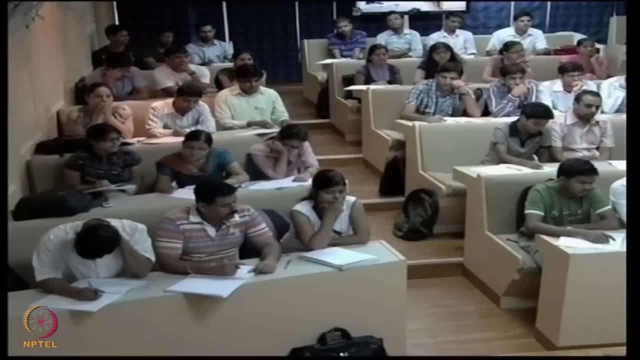 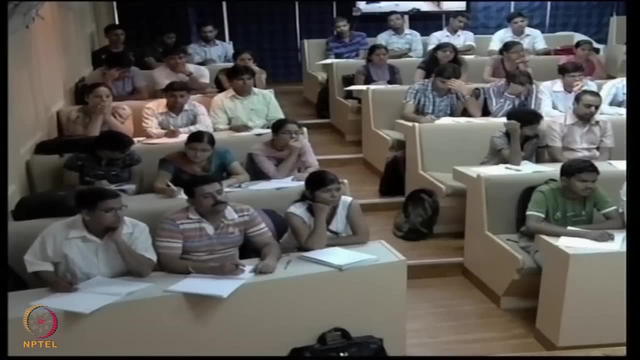 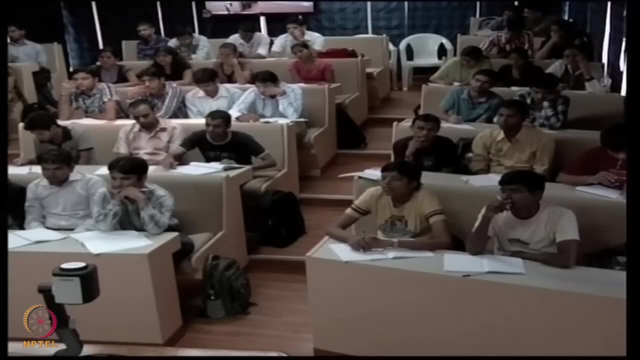 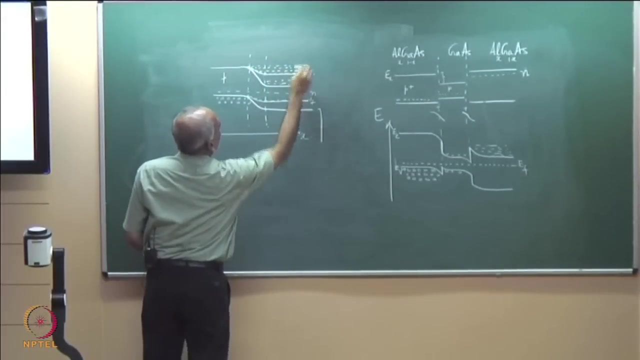 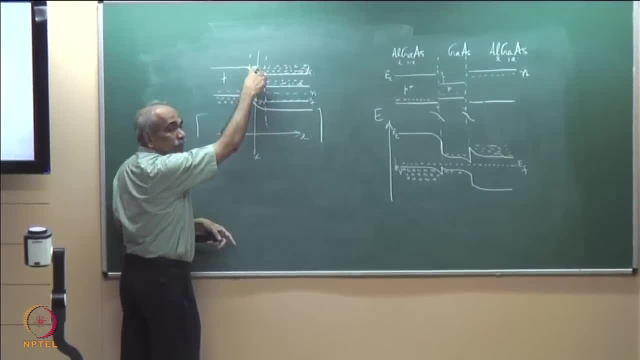 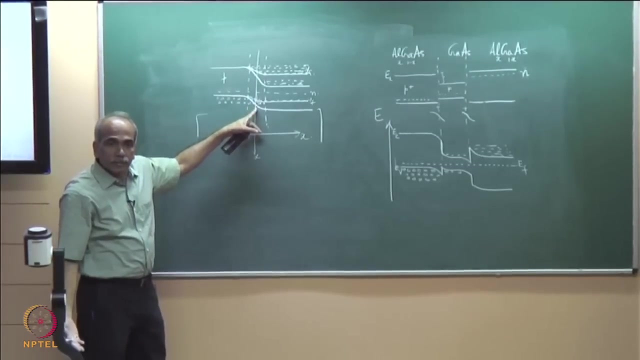 you have simultaneously large number of holes and large number of electrons. Earlier in this junction region you did not have electrons and holes. Now you have large number of electrons and large number of holes which recombine to form the current, So you have forward bias. 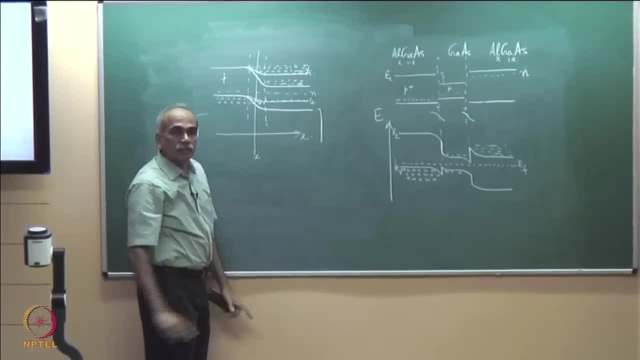 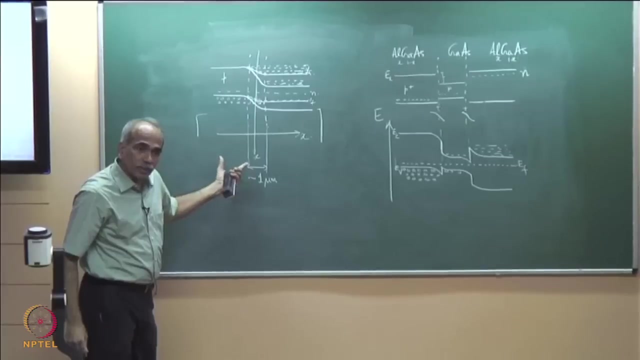 therefore the carriers recombine and current flows in the external circuit. This is how the p? n junction would work. But this region, this variation here, is approximately 1 micrometer in typical semiconductors. The width of the depletion region, of course it depends on the doping concentration. If you, if the doping concentrations are high, there will be a decrease in the concentration. If the concentration is high, there will be a decrease in the concentration. If the concentration is high, there will be a decrease in the concentration. If the width of the depletion region is small and the field is very high, 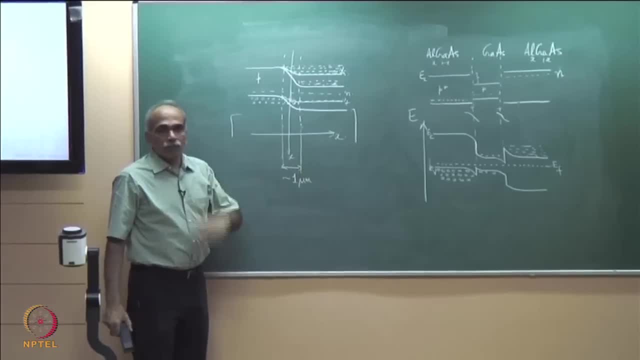 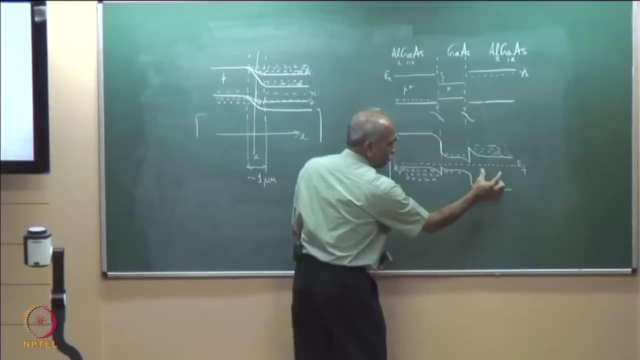 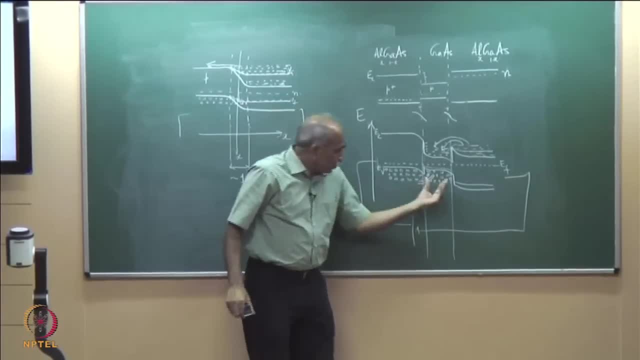 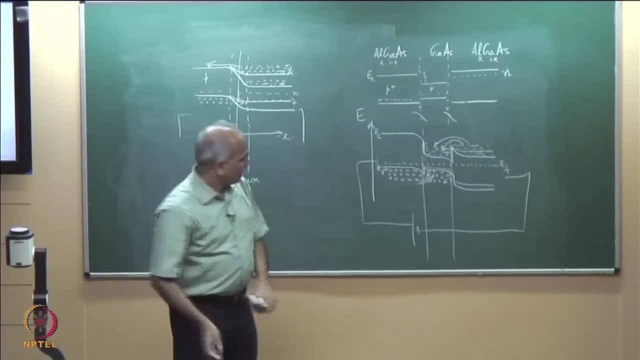 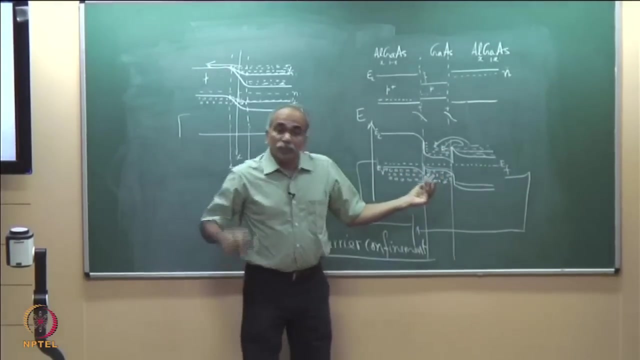 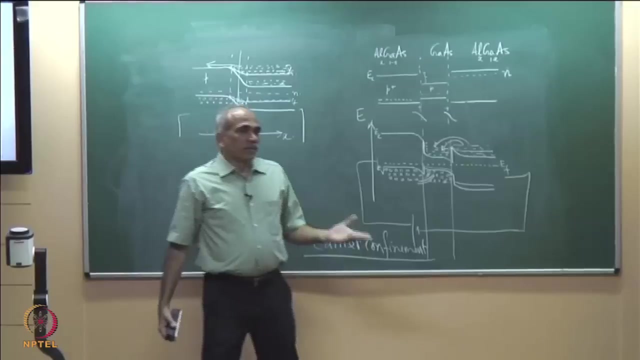 important advantage of heterostructures. this is called carrier confinement. there are other advantages we will discuss later. so what is the point? for the same current, you have very large number of carriers in a small volume, which means the carrier density is very high. as we will see later, the gain of the medium is dependent on carrier density. 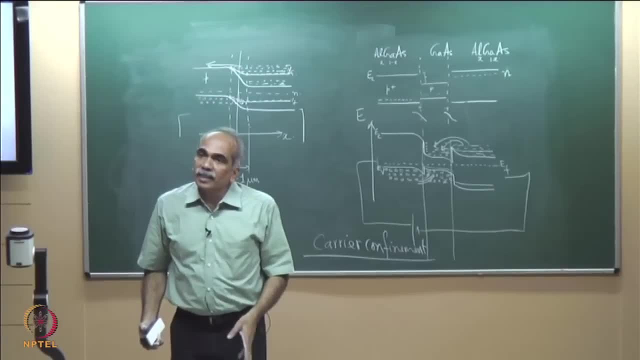 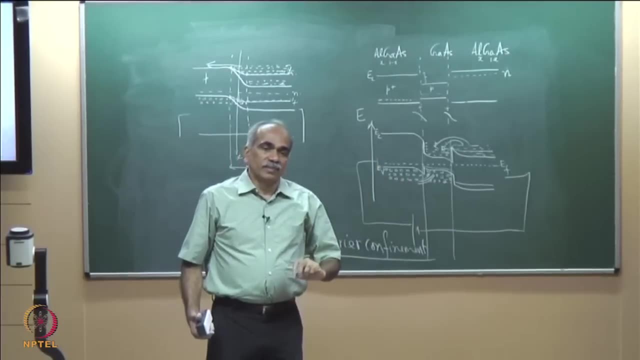 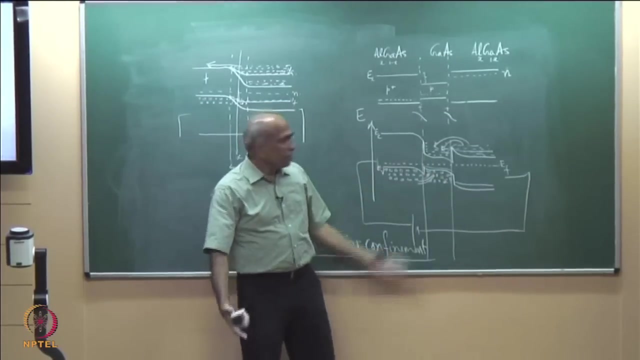 So if you can have a large carrier density for a small current, you can get very high gain for a small current. this is the importance of double heterostructures. therefore, if you understand this band diagram and see that how the discontinuity helps in confining the 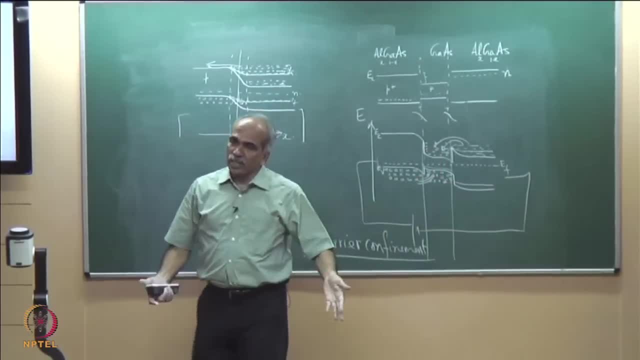 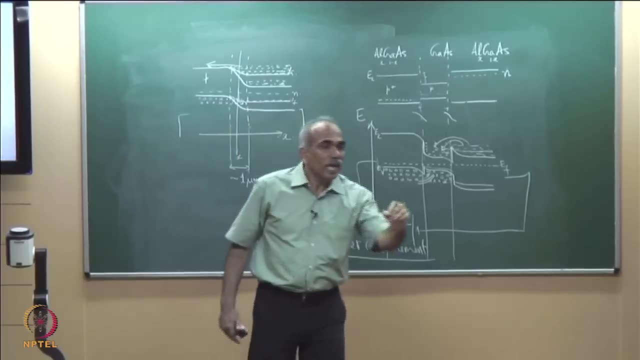 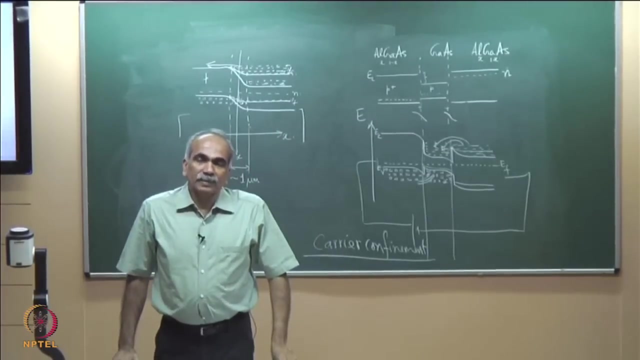 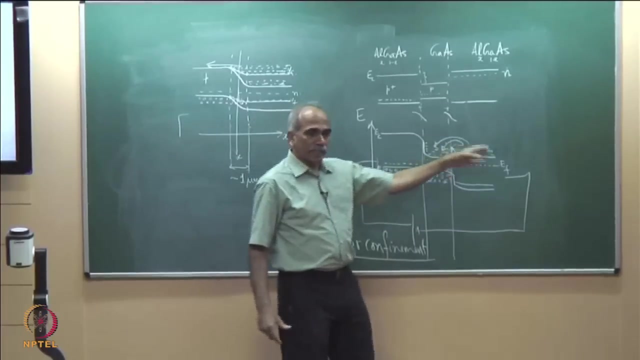 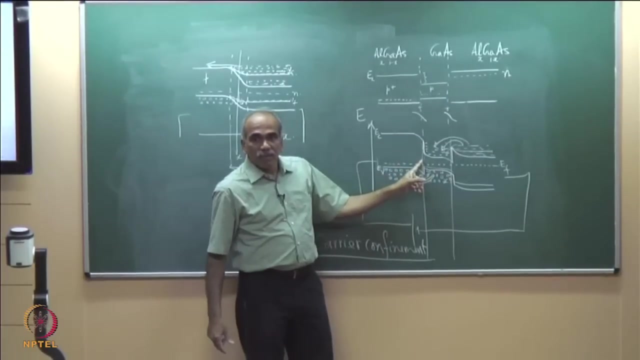 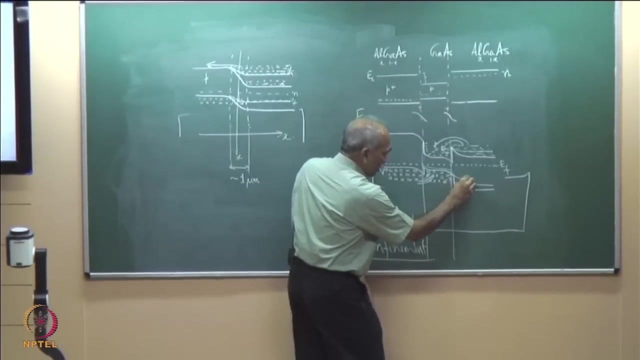 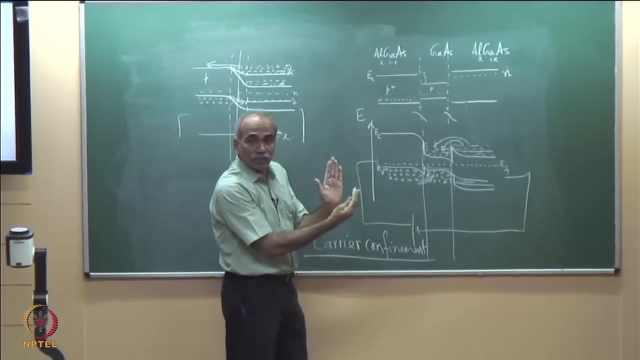 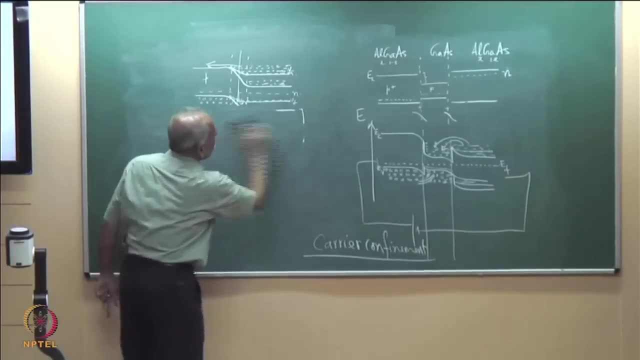 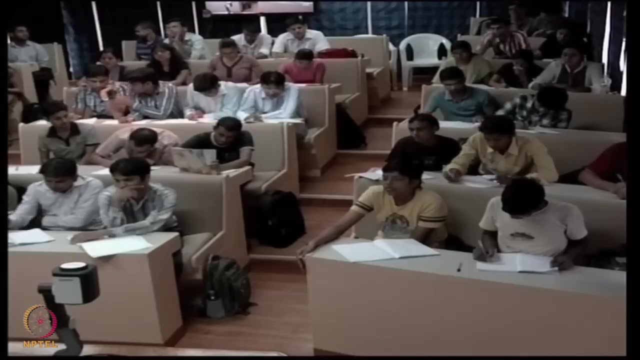 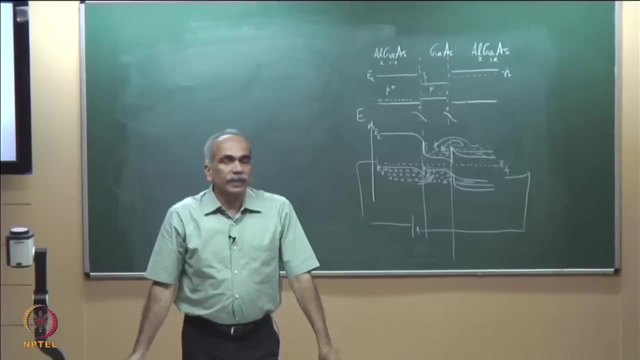 carriers, then you can appreciate that the discontinuity I have illustrated for a double heterostructure. in the next class we will discuss about short key junctions and ohmic contact, the last of the basic topics which are required to understand the device. physics device.